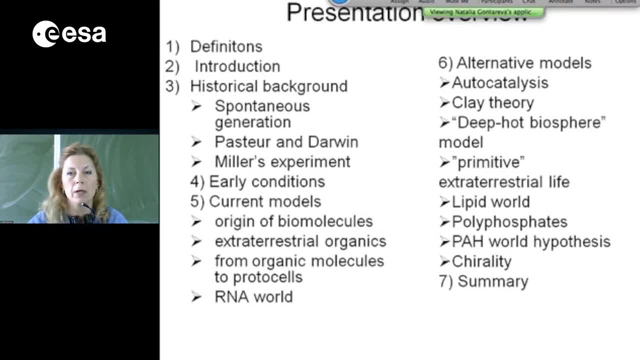 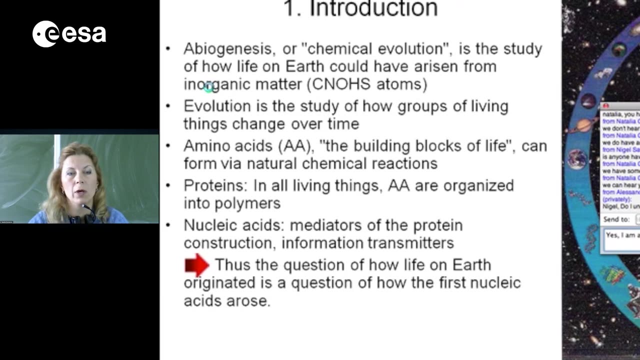 Also, then I would like to speak about some alternative models of life origin, And then I will give you a short summary of the presentation. So, first of all, we should figure out what is chemical evolution, And right now it is supposed to be the study of how life on Earth could appear from non-organic matter. 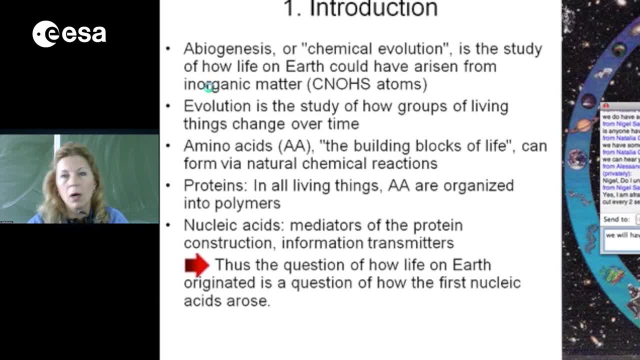 And the main atoms which took part in the appearance of the living system are carbon, nitrogen, CNOHS, And the building blocks of life are mainly amino acids. Then the monomers of amino acids are polymers of amino acids are proteins. 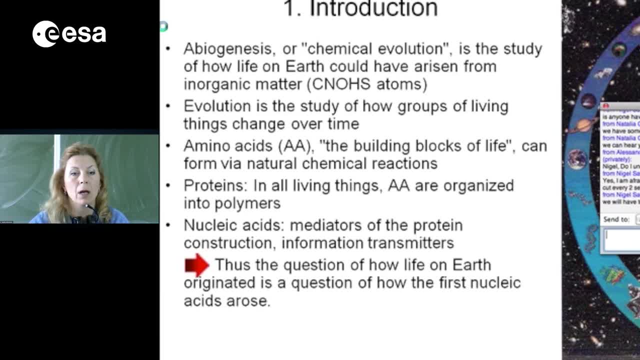 Then nucleic acids, which are mediators of the protein construction and information transmitters as well. Of course, we will speak about lipids, who are structural units of any living cell, And generally discussion about the structure of living cells. And of course, we will talk about the structure of living cells. 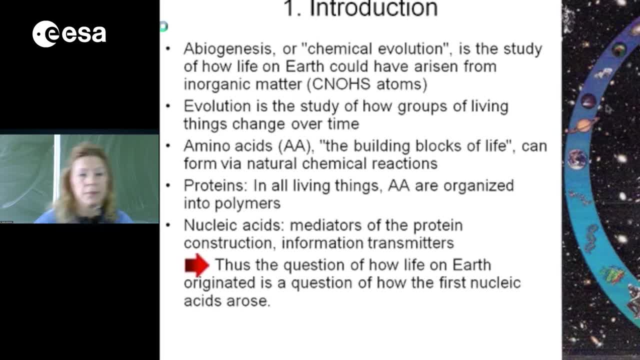 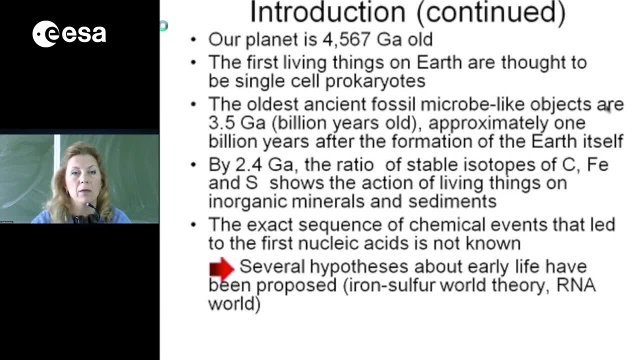 And of course, we will ask the question of how life originated. So it could be a question of how the first nucleic acid arose. As we already heard from Alexander's presentation, our planet is more than 4.5 billion years old. And the first living things found on Earth are supposed to be single celled prokaryotes. We can also date the oldest ancient fossil. It is as old as 3.5 billion years old. We can assume that the life on Earth, or at least first living systems, appeared quite quickly after the formation of the planet itself. 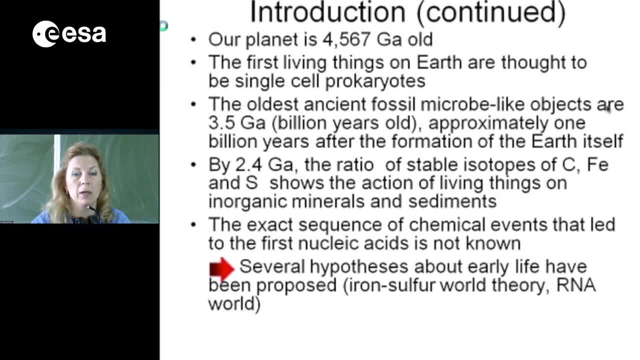 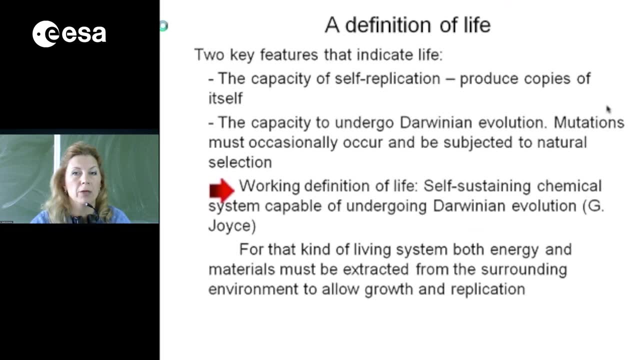 So the question is: what sequence of chemical events led to the first living organisms? What happened? What happened? Why did it appear so quickly? I would like to give the definition of life as a living matter. So, first of all, there are two key features that are typical for living systems. 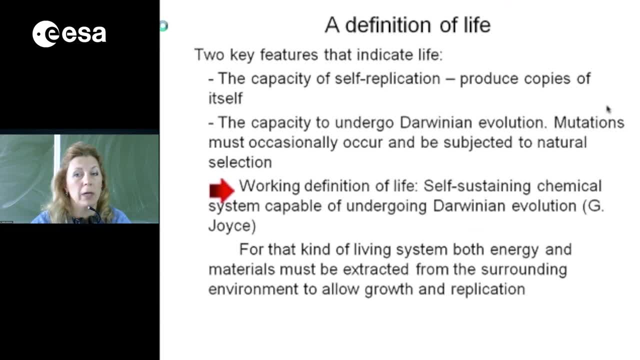 First of all, it is the capacity of self-replication. So living organisms, whether it is a cell or a big organism, should be able to produce copies of itself. Then these copies should evolve. They should not stay as they were initially. 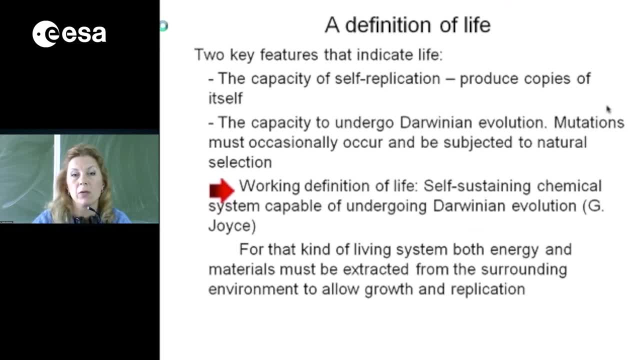 So this is the capacity to undergo Darwinian evolution. So these organisms and these systems should be subject to natural selection. improving the the initial choice of improving the natural initial situation, The working definition of life is the self-sustaining chemical system capable of undergoing Darwinian evolution. 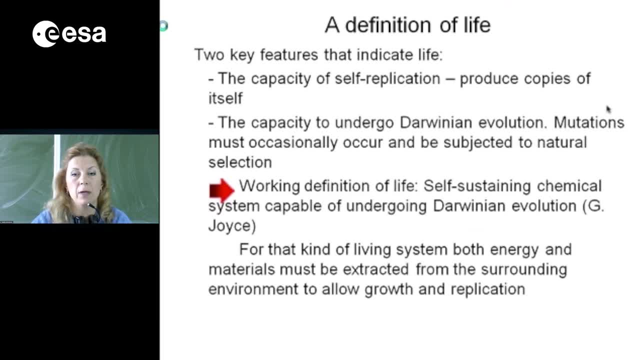 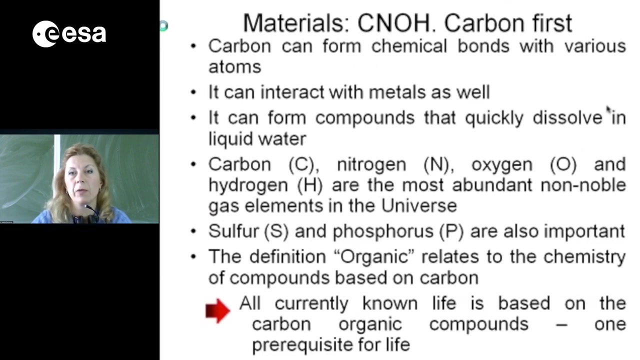 To proceed with this evolution we need to have energy, materials and some exterior, some surroundings that let cells or molecules to grow and to replicate. First of all, materials. What do we need for construction of primitive cells? It is the same material for both human organisms and bacteria. 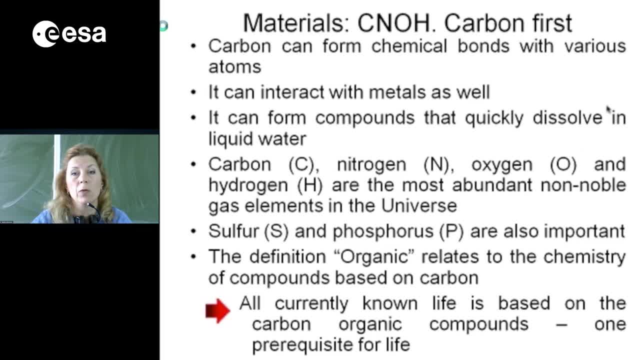 It's first carbon, which is one of the most abundant elements in the universe and on Earth as well. So it's unique because it has certain properties. Carbon can form chemical bonds with various atoms. Thus it is able to shape up as different molecules. 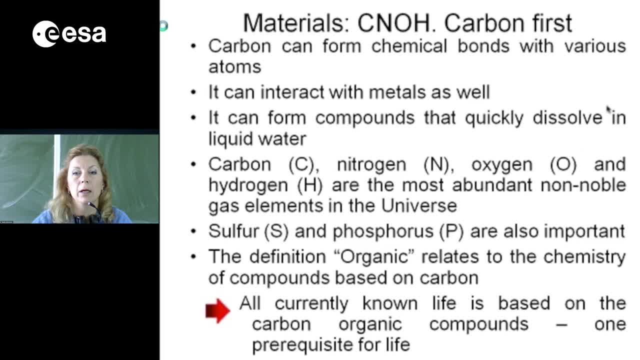 It can interact with metals and its derivatives are soluble in water. in liquid water, Apart from carbon, we have nitrogen, oxygen and hydrogen, which are the most abundant non-noble gas elements in the universe. We should also mention sulfur and phosphorus. 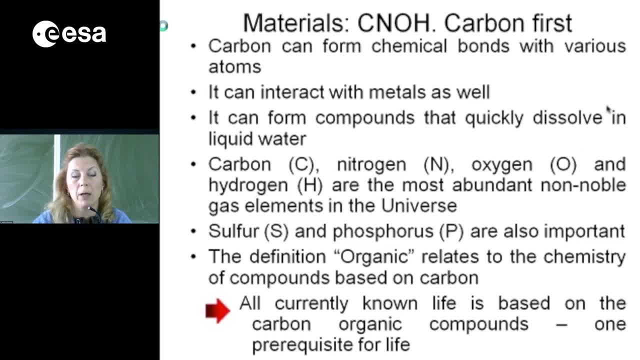 which are important and which are the compounds of biological molecules. So at present time we know only organic life based on carbon, And all currently known theories take carbon derivatives as its base. It's one of the prerequisites of life: The presence of carbon. 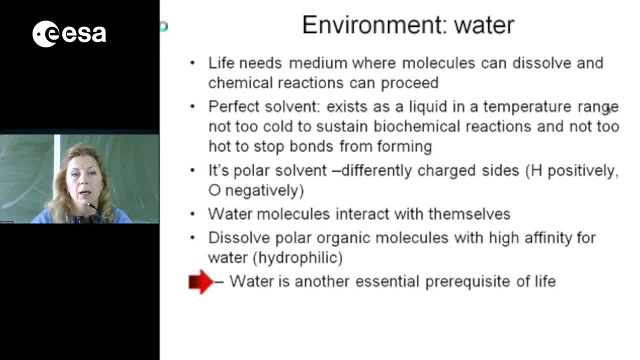 Then the environment. Life needs some medium where molecules can move, can dissolve and can interact. So water, in this case, is a perfect solvent. It has a wide temperature range where it exists as a liquid, So it's not too cold for biological biochemical reactions. 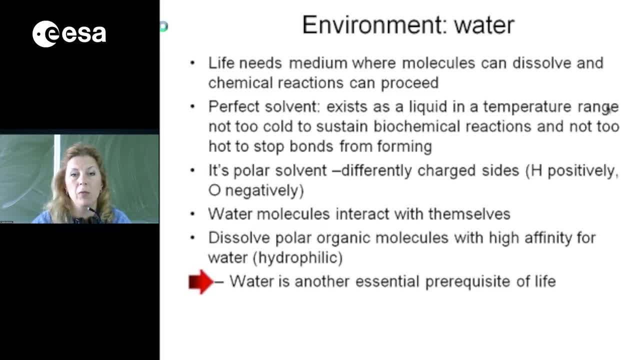 and not too hot to destroy. It's a chemical bond. Besides, it's a polar solvent. It has differently charged sides. You know, one is charged positively. The molecule of water dipole Water molecules. they interact with themselves and dissolve polar organic molecules with high affinity. 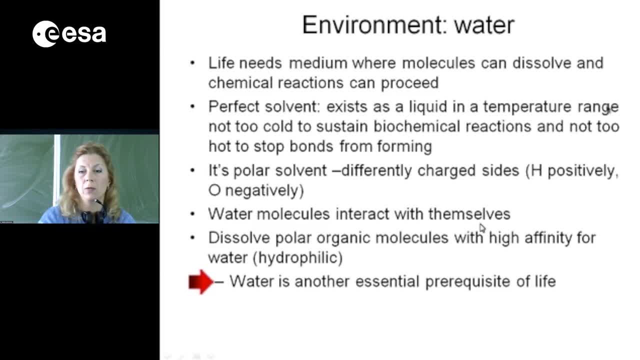 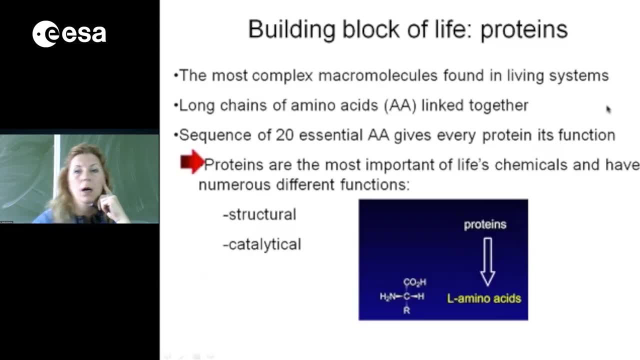 So we can conclude that water is another important prerequisite of life. Then number three: building blocks of life: What do we need to construct cells? Proteins First of all. it's the most complex macromolecule molecules found in living systems. 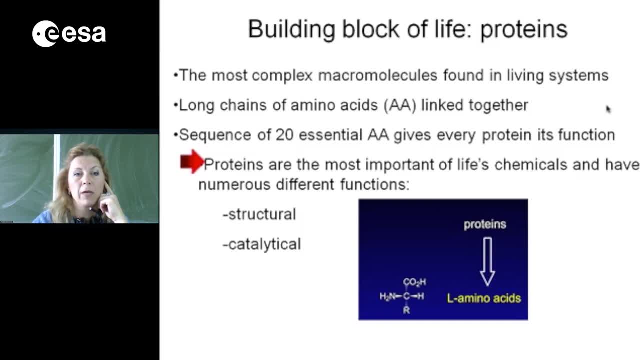 They actually represent long chains of amino acids linked together, And the sequence of amino acids of 20 main amino acids give every protein its function. So the function of a protein appears due to the sequence of amino acids. We can say that proteins are one of the most important of life chemicals. 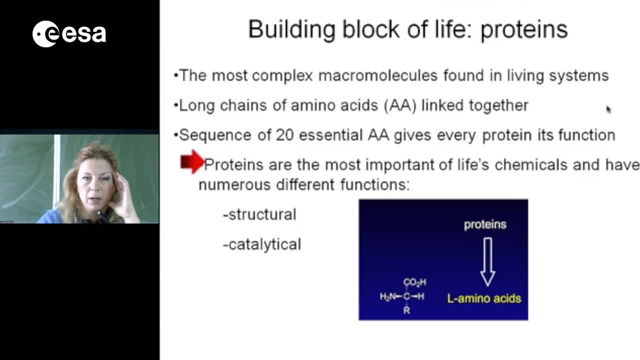 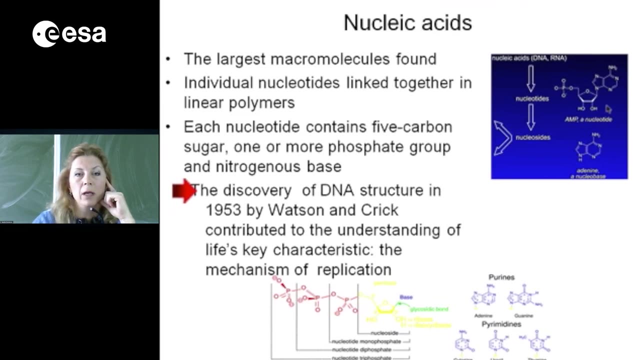 and have different functions, just to name structural and catalytical. Then nucleic acids. These are. these molecules are much bigger than the amino acids And they represent individual nucleotides linked together in linear polymer, long chains of polymer. Here we have some picture to so you can see the structure of nucleotides. 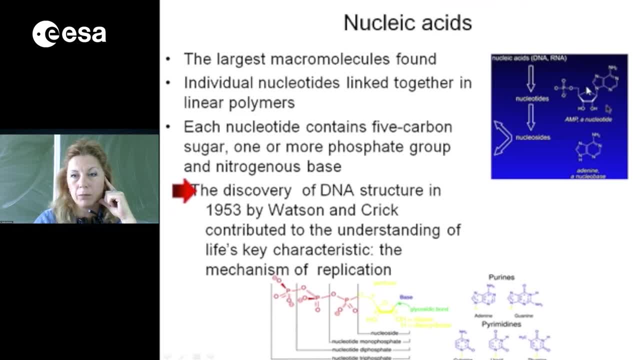 So it consists of a base, of a phosphate group and the sugar. So this is the base. So this: each nucleotide contains five carbon sugars, one or more phosphate groups and nitrogenous base, And the most important discovery in this area was the structure of DNA. 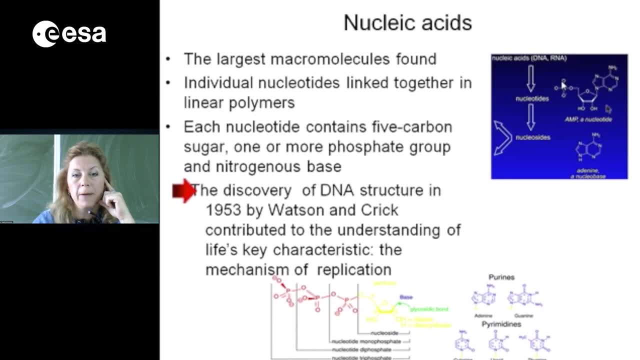 which was revealed by Watson and Crick in 1953.. And it helps to understand the mechanism of replication. So in the lower part of the screen you can see the picture where three phosphate groups are linked together to the nucleotide, So nucleotide, then one phosphate group is nucleotide, monophosphate. 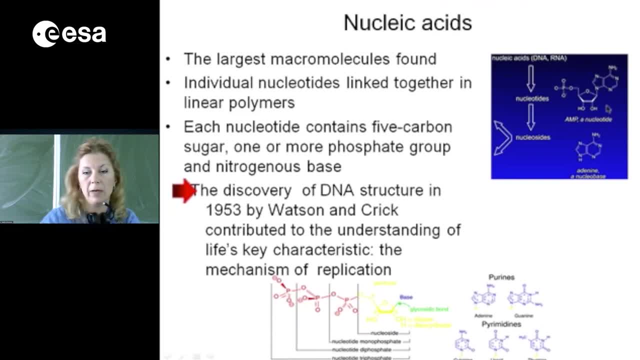 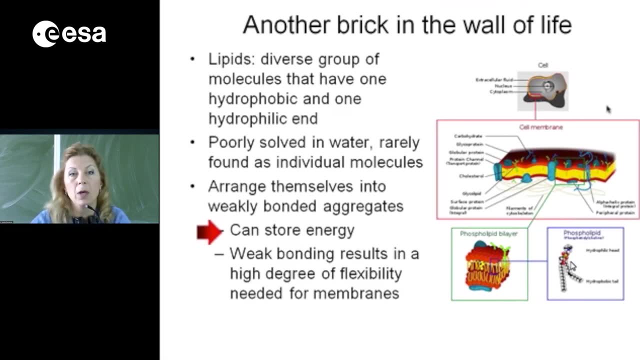 then diphosphate and triphosphate. Here are the bases. We should also mention lipids, which are the diverse group of molecules. They have one hydrophobic and one hydrophilic end, And this structure lets them to be organized as layers. 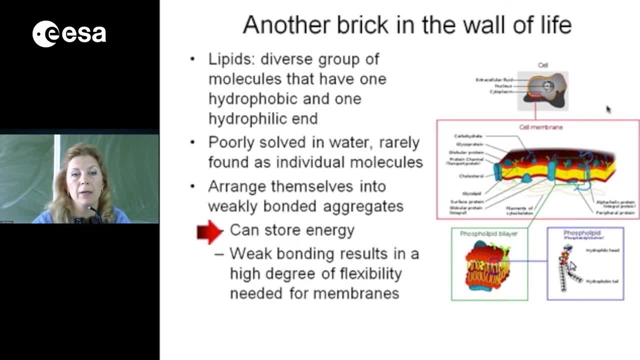 They are poorly sold in water and they come as aggregates, not as individual molecules. So properties of lipids are that they can store energy and they have weak bonding in between. So it results in a high degree of flexibility, Which is quite useful for construction of membranes. 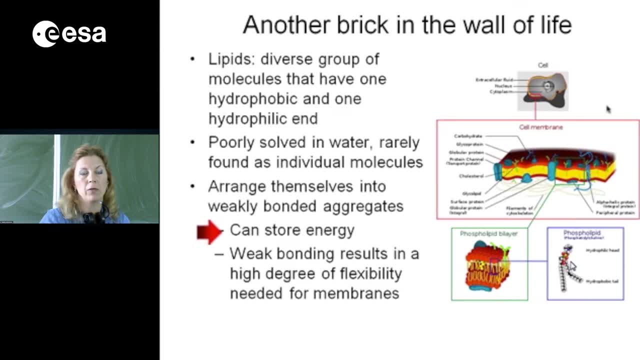 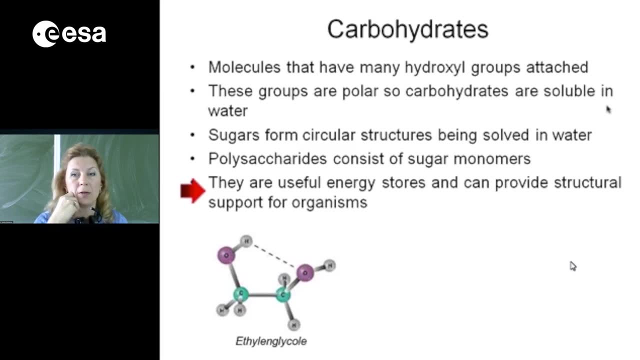 I mean membranes of living cells, Carbohydrates, sugars, Molecules that have many hydroxyl groups attached, and these groups are also polar, And this molecule is soluble in water as well. Polysaccharides consist of individual monomers, and they are also used as energy storages. 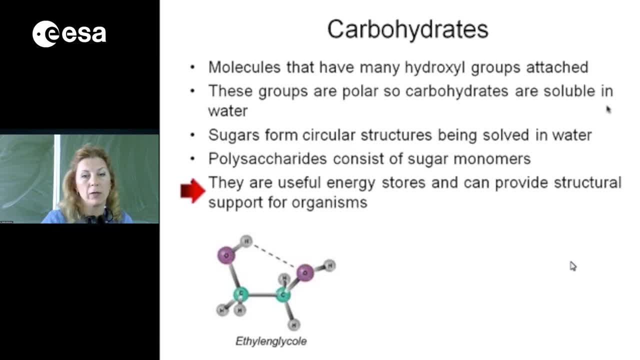 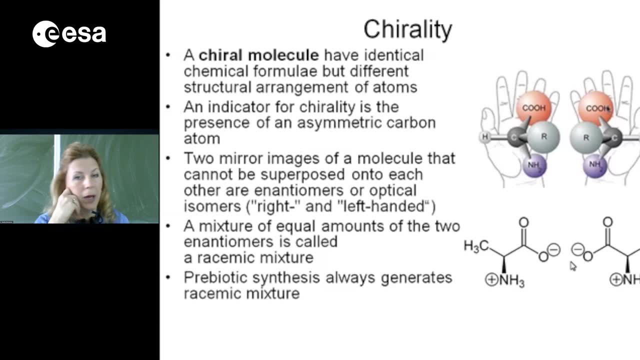 and can provide, besides, structural support for organisms. Sugars are also included in nucleotides. I would like to say a couple of words about chirality, Although this is a very big topic which cannot be revealed in a structure in a frame of our lecture. 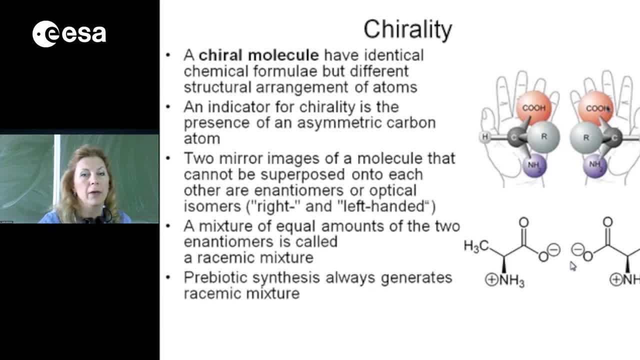 So these are chiral molecules. They have identical chemical formula but different structural arrangements, So they are shaped up like two hands. And in living systems only one type of molecules are used, At least of amino acids. Usually if you go to a chemical mixture. 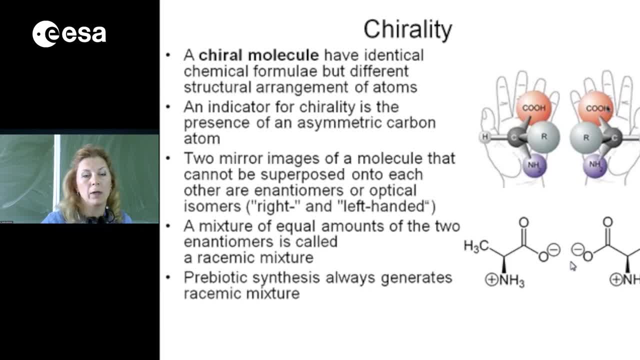 it will be a racemic mixture. So where it's a, Where proportion of L and D forms is almost equal, And prebiotic synthesis will provide a racemic mixture, but not in nature. In nature, one form dominates the other. 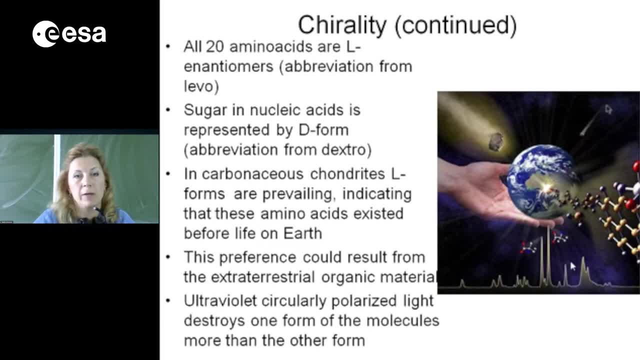 As I told you, all 20 amino acids which are used in living cells in structures are L forms, While sugars, for example in nucleic acids, are D forms In the extraterrestrial material found, for example, in meteorites. 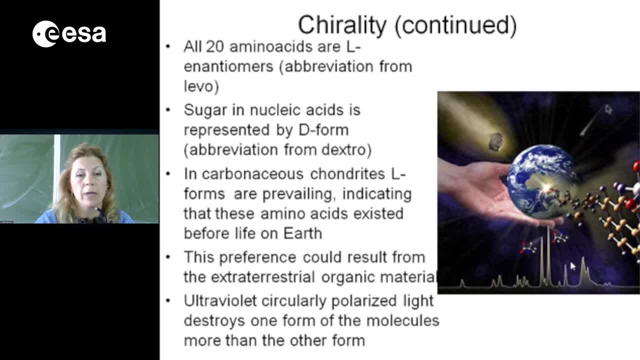 carbonaceous chondrites, scientists found L forms prevailing And this is an indication that life in general, at least those living forms, existed before life on Earth. So there are several ideas of how these different shapes of molecules could appear, how they could evolve. 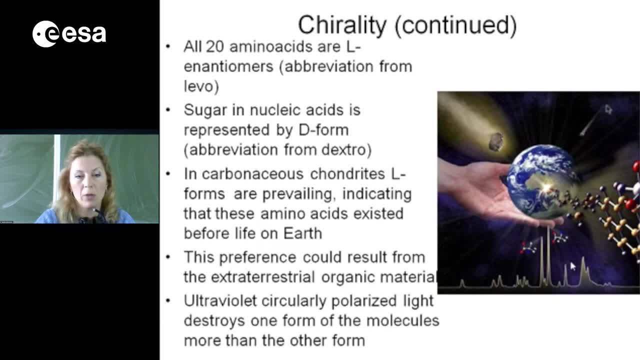 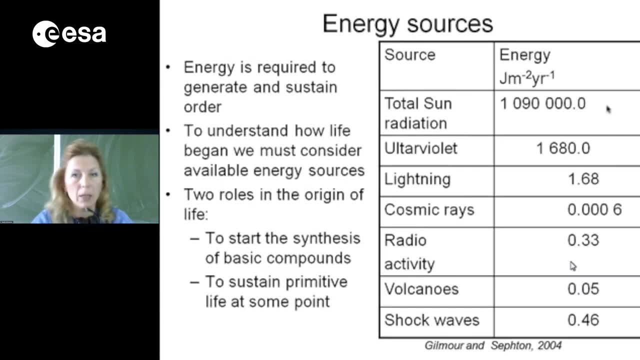 And one is that this is the result of action of ultraviolet polarized light, circular polarized light. Then, to construct some chemical reaction, to start it we definitely need certain energy impact, And we can think about energy sources that are currently present in. 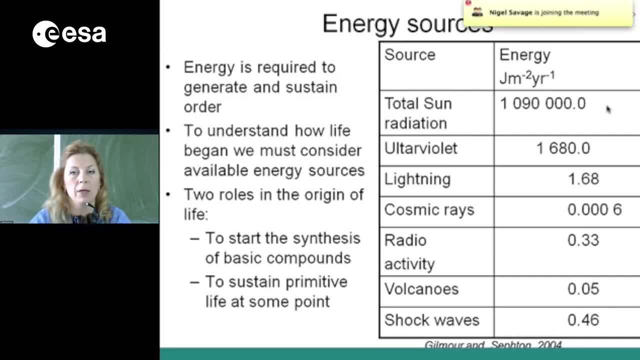 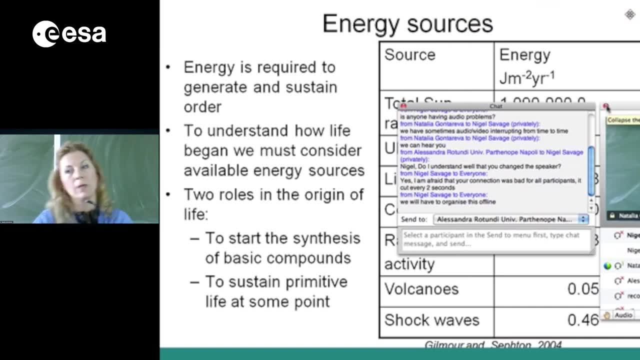 for example outer space, and that were present on the primordial primitive Earth. So total sun radiation is the prevailing source of energy And it consists of ultraviolet, which is quite important. It is sufficient in biological reactions. Also, lightning provides the energy of these charges. 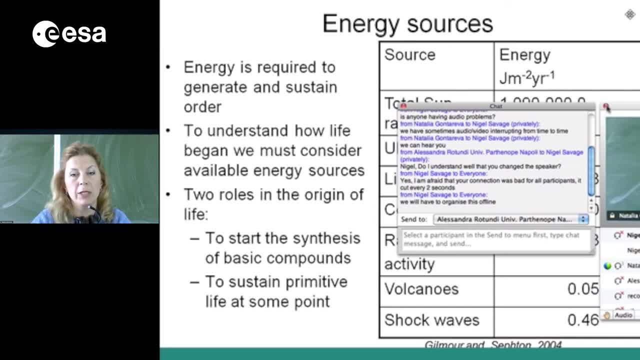 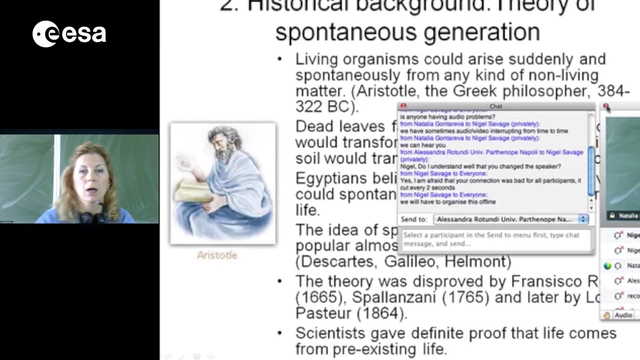 And we have cosmic rays and radioactivity, external and internal, In the primitive Earth, for example during the volcanic eruption. volcanoes provide a certain amount of energy And shock waves as well, after meteorite impacts, for example. In the historical background. 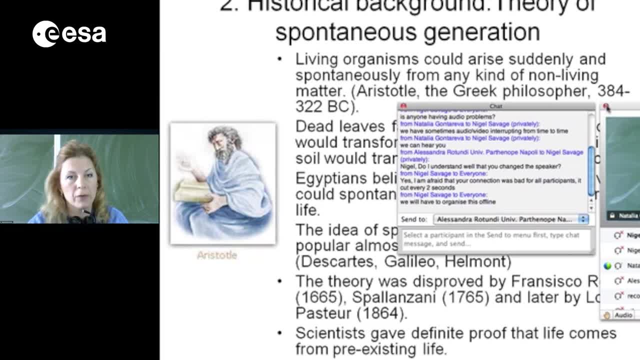 there were certain theories which tried to describe how living organisms appeared And if we go back to the history, to Aristotle, for example, he supposed that living organisms appeared suddenly and spontaneously from non-living matter. So the idea that living matter is related to non-living matter. 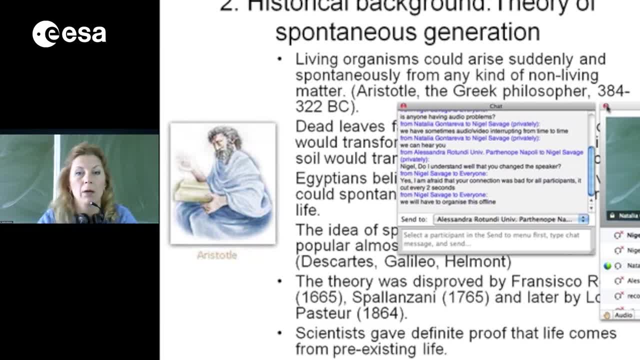 is already quite old. Examples were dead leaves falling from the trees then later turned into fishes, And those leaves who were on the soil transformed into insects and some worms. Egyptians who were very much fond of the river Nile. they believed that everything originated. 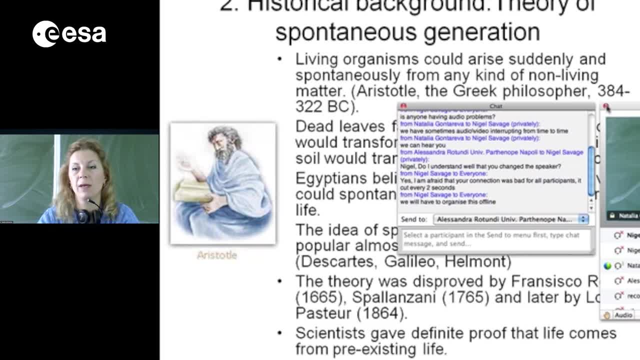 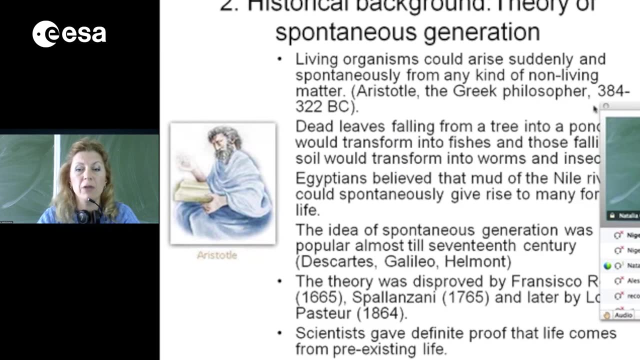 from the mud of the Nile River. So Nile was the beginning of everything, And this idea of spontaneous generation was quite popular until the 17th century, And it was disproved later due to the experiments of Louis Pasteur, Francesco Redi. 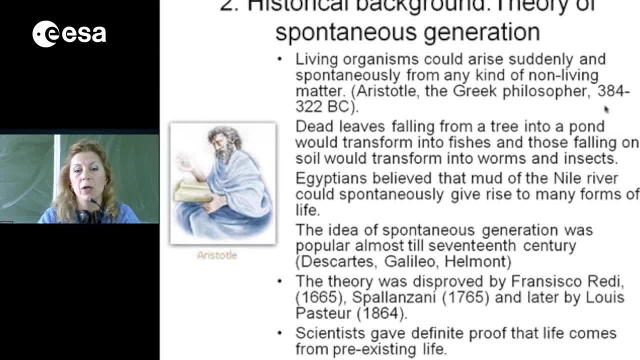 Polanzani and many other researchers who showed that it is not possible. So to start to produce something, you should have some basic materials. So scientists gave definite proof that life comes from pre-existing life. just forms are different, As I told you. the works of Louis Pasteur. 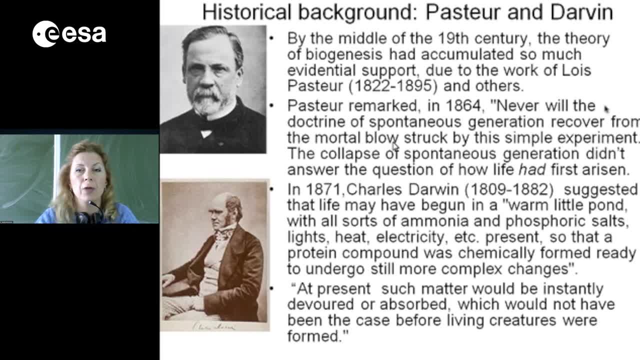 contributed greatly to destroy this theory of spontaneous generation. And Pasteur noticed that the collapse of spontaneous generation didn't answer the question of how life had first arisen. It was just the consultation of facts that it appeared from this to this, but it didn't give any explanation. 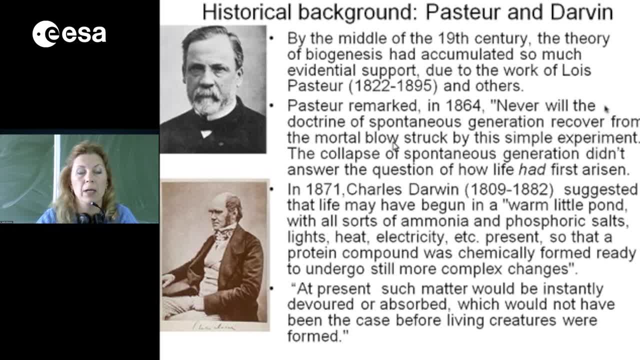 Charles Darwin proposed his theory in 1871, which is very much similar to what we think now. So life appeared in a warm little pond enriched with ammonia, phosphoric salt, having energy in forms of light, heat, electricity, so that protein was chemically formed. 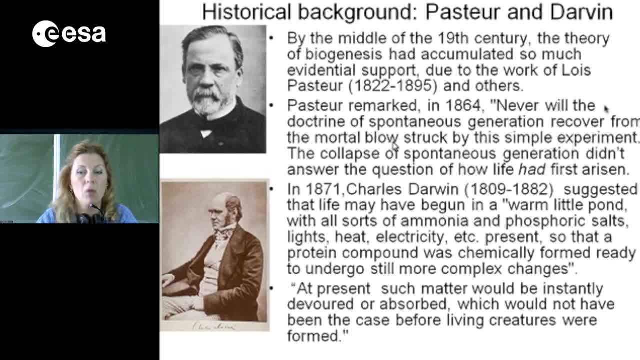 and then able to undergo still more complex changes. So this is actually the formulation of evolution theory. Right now, such a matter would be instantly destroyed, But before that, where there was no living creatures, that was quite possible. So human beings are the most destructive. 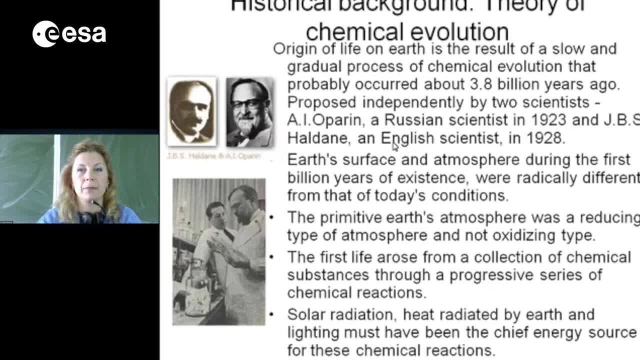 factor right now. Later on, this theory was proposed independently by two scientists, Alexander Aparin in 1923 and Holden, an English scientist, in 1928.. And we should mind also thinking about this theory that at present time. 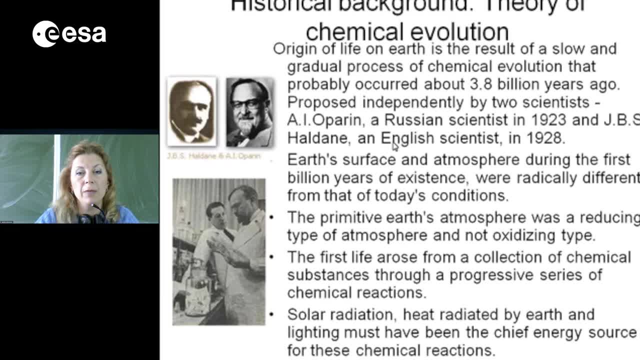 at the early Earth surface and atmosphere during the first billion years of its existence were different from what we have today. So the primitive terrestrial atmosphere was a reducing type, not oxidizing, And Aparin thought that first life arose from a collection of chemical substances. 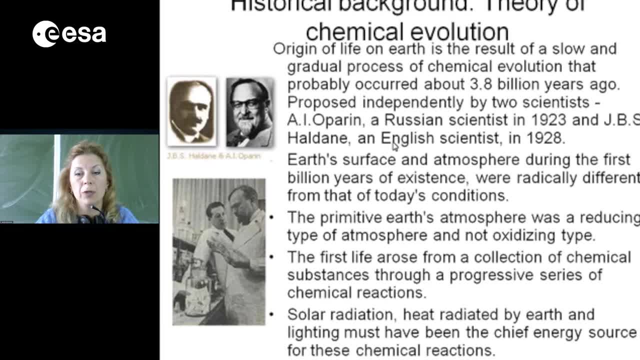 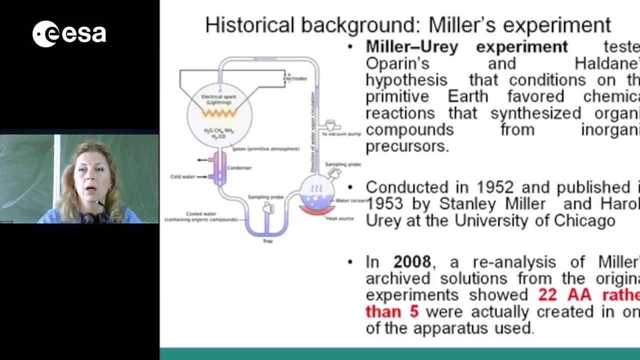 which were able to undergo a progressive series of chemical reactions, And solar radiation and heat were used as chief energy sources for these chemical processes. So this theory was later on tested by Miller- Stanley Miller, who was an American scientist- And he did a very simple 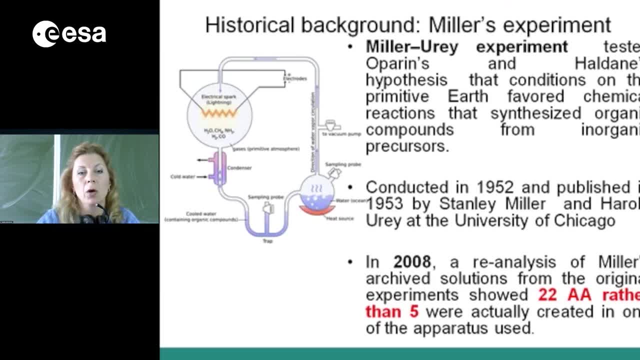 but very effective experiment, And he was able to show that genius is thinking simple. So it was published in 1953. And the experiment included glassware where chemical ingredients were added as gases like H2O, CH4, NH3,. 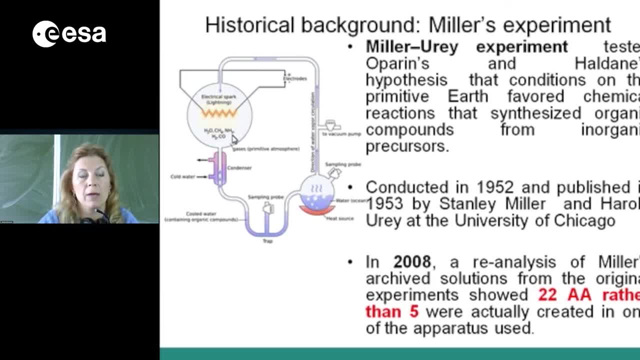 and electrical discharge was used as a source of energy, so simulating lightning, And then the derivatives were arriving to the reservoir, where they were later on analyzed. What is interesting? that in 1928,, I'm sorry, in 2008,. 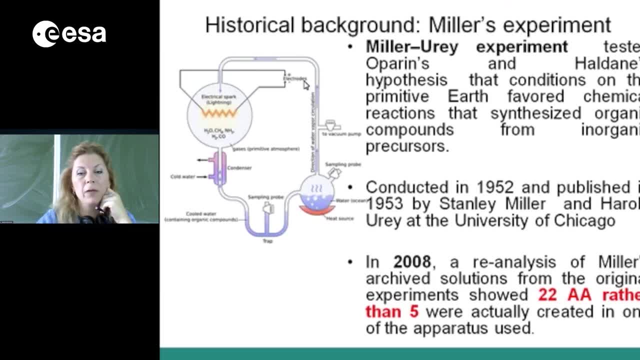 it was a reanalyzing of Miller's experiments, because they managed to find in archives several solutions from Miller which were not analyzed before and they were kept for many years. So Stanley Miller: he found five amino acids And then in 2008,. 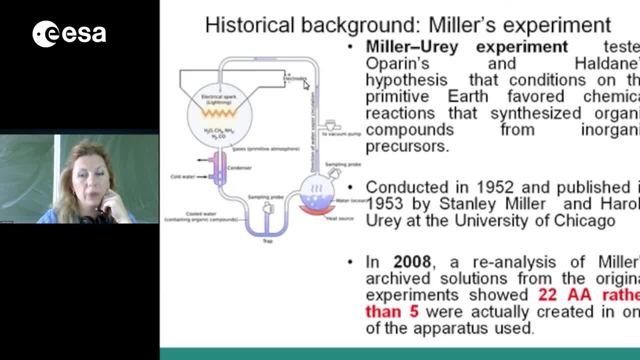 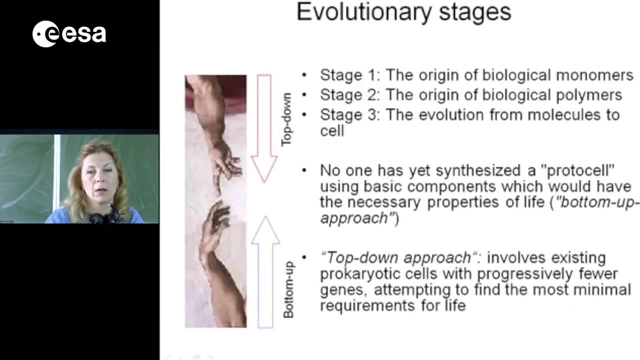 there were 22 amino acids extra. So actually during that time, in 1953, he was not able to detect the whole range of products. but it was done later on with a big success. So now we will proceed to the theories. 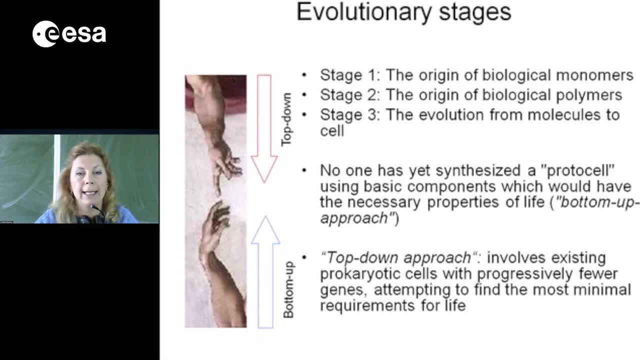 And I would like to show you this slide to speak about two kinds of approaches. So there is a top-down approach from top to bottom and bottom-up approach, from bottom to top. So top-down approach means that you take existing cells and then to take away. 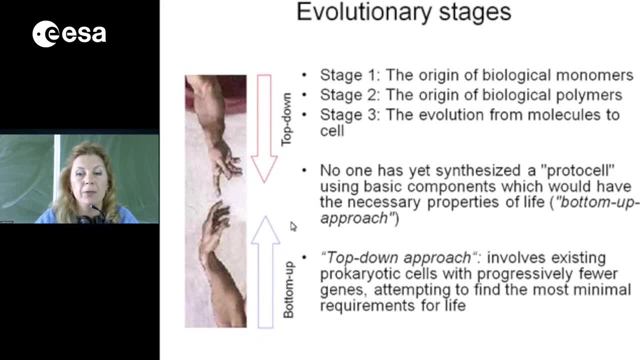 several genes from it, attempting to find the most minimal requirements for life and then to base your presumptions on these experiments And bottom-up approach is to having no. sorry, it was a bottom-up approach, So it's having a protocell. 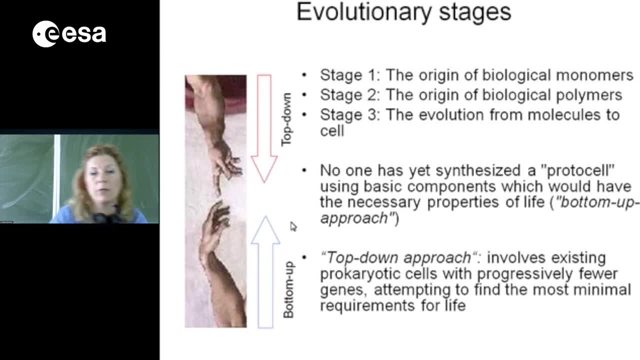 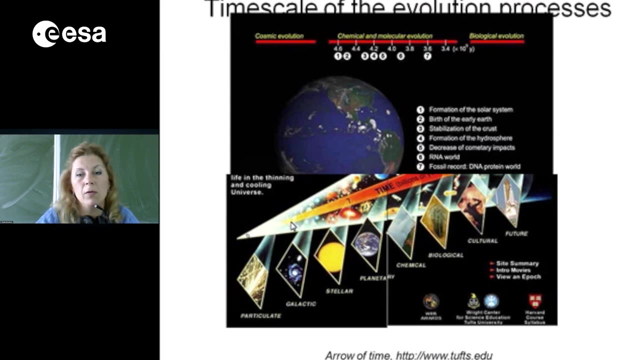 using basic components which have the necessary properties of large of life. So both approaches are equal and they none of it is prevailing. This is also the timescale of evolution. I already mentioned several figures and we know that life, that our planet, existed. 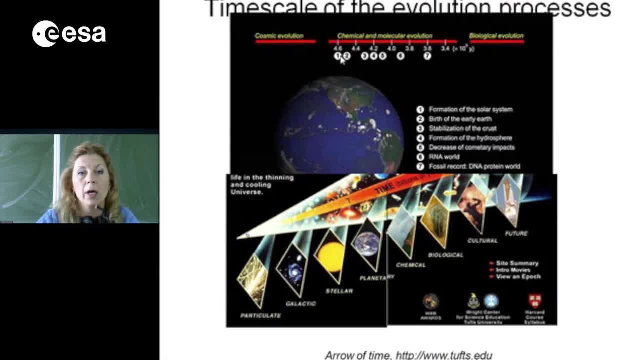 4.5 billion years ago. And chemical. we think we presume that chemical and molecular evolution started by that time. Then it was followed by biological evolution and it was preceded by cosmic evolution. So the first fossil records, the first living systems. 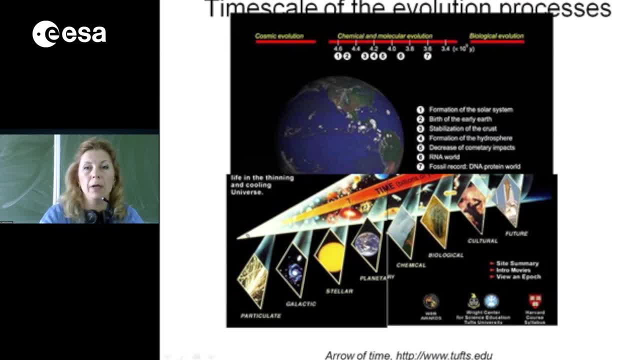 were already appeared 3.6 billion years ago. That's why the period of appearance of life is quite short. It should be some reason for that phenomena. Why did it happen so quickly? That's why scientists and people in general are trying to think about it. 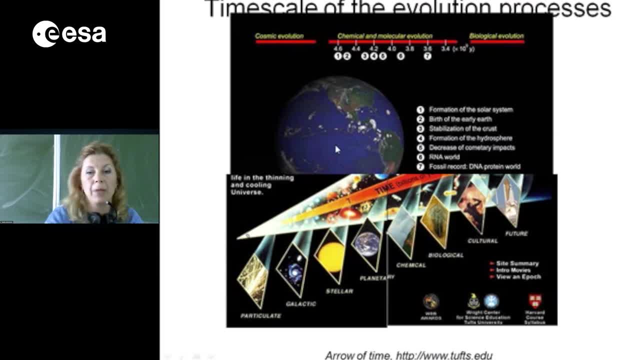 all the time, And that's why this question is so important. At the bottom part of this slide you can see a bigger scale. So chemical evolution is just a part of this small arrow of time. I like this very much. I think it's very. 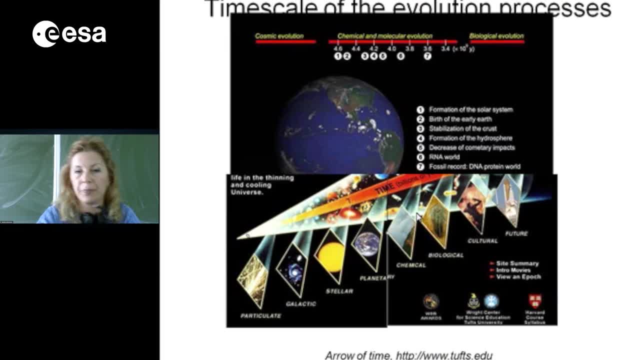 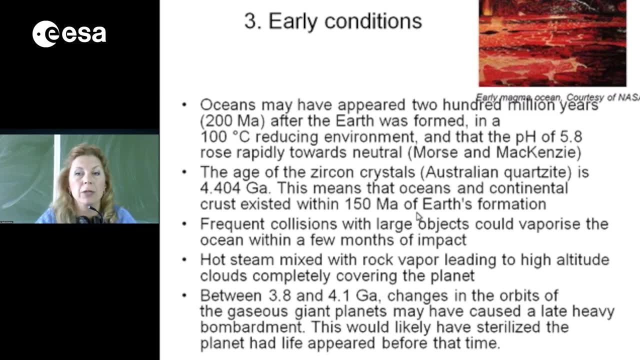 it's showing very good how everything happened and what will be next, what will come next. So oceans might have appeared about 200 million years ago, right after the Earth was formed, in a quite hot and not friendly environment, And we know that there was a period of 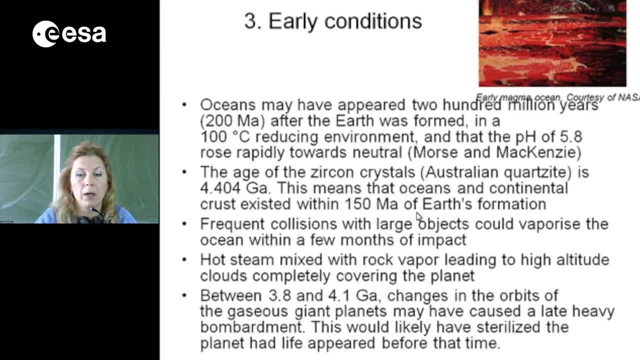 intensive bombardment during the history of the Earth formation During this bombardment time. it's very likely that if there were any organic matter before that, it would have sterilized the bombardment. It would have sterilized the planet if life had appeared. 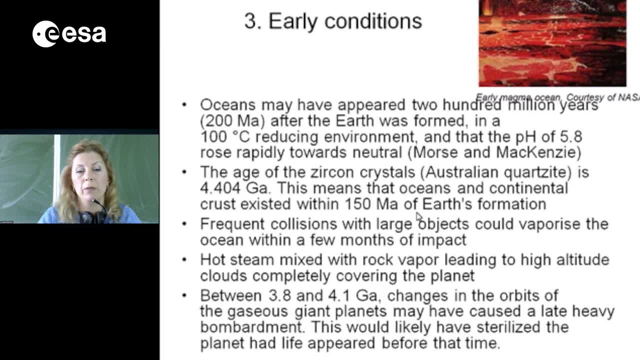 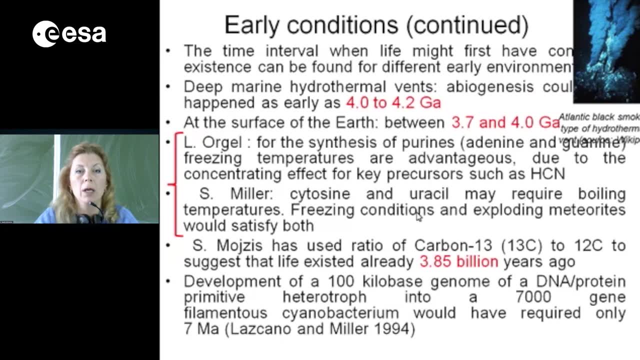 before that. So the period is actually even shorter, starting from 4.1 billion years. Then if, to speak about early conditions, we have deep marine hydrothermal vents which have conditions very favorable to formation of organic matter. So in this environment, 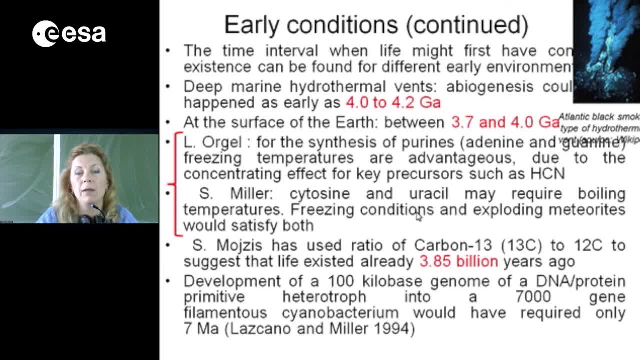 life could have appeared as long as 4.2 billion years ago. Then we have a surface of the Earth. now we are talking about primordial Earth, primitive. The conditions were different, but they could suit different types of molecules, For example. synthesis of purines, it require freezing temperatures, while the synthesis of another citizen and uracil may require boiling temperatures. So it's different conditions, but they also existed. For example, you can think about exploding meteorites and freezing conditions in the polar region. 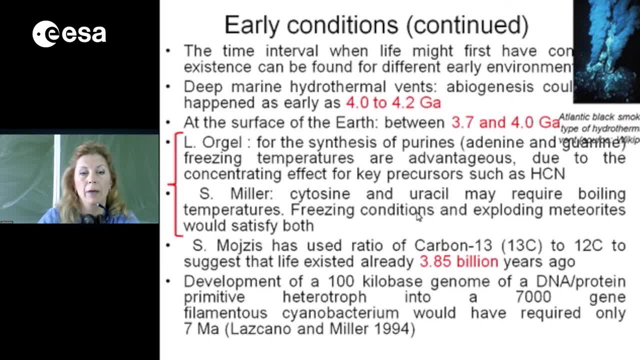 There were also other indications that life existed already quite long ago, For example, ratio of carbon-13.. And then if to think how much time is needed for develop 100 kilobase genome, for example of DNA and the DNA of the human body. 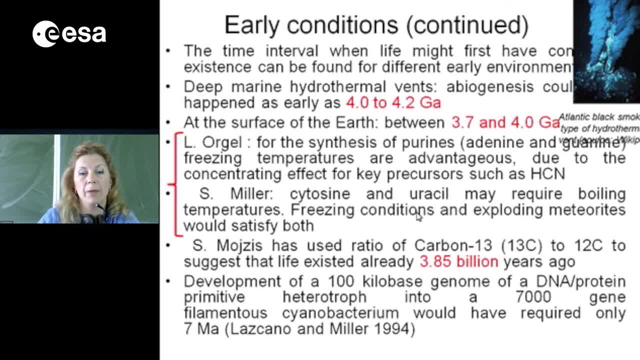 And then if to think how much time is needed for develop 100 kilobase genome, for example of DNA protein, into 7,000 genes of cyanobacterium, it would have required 7 million years. So the early atmosphere. 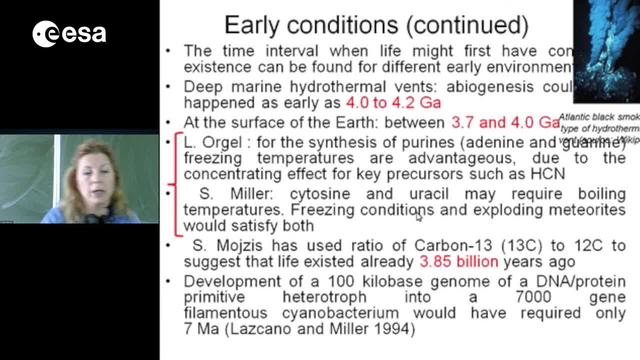 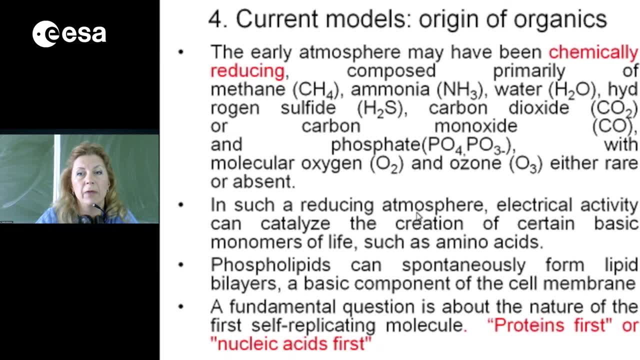 may have been chemically reducing, and it consisted of several types of gases: Methane, ammonia, water, hydrogen, sulfide, carbon dioxide and the carbon dioxide that is present in the atmosphere of the human body, And then, of course, the 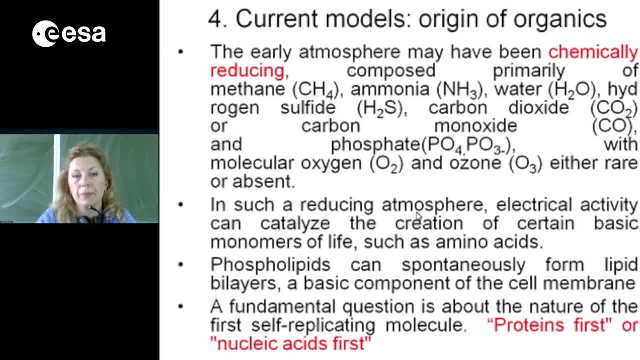 carbon dioxide or monoxide and phosphate. Of course, molecular oxygen and ozone were quite rare or absent. This was a reducing atmosphere and in this atmosphere we needed some electrical activity to catalyze the creation of monomers. Monomers are the first self-replicating. 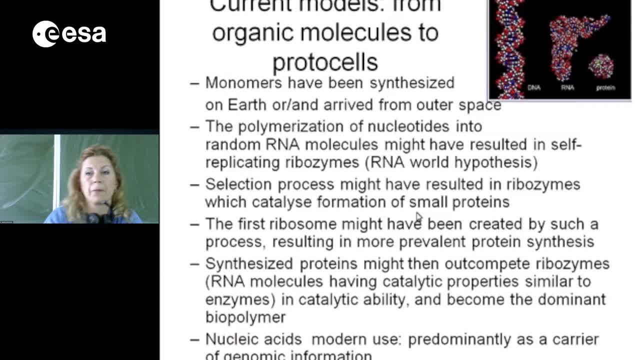 molecules. So what happened first? Proteins first or nucleic acids first. So if to go, if to see about the difference between RNA, DNA and protein, both DNA and RNA are quite long and they can be synthesized on the Earth on. 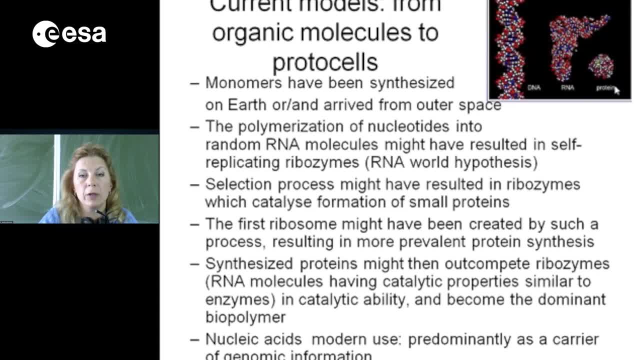 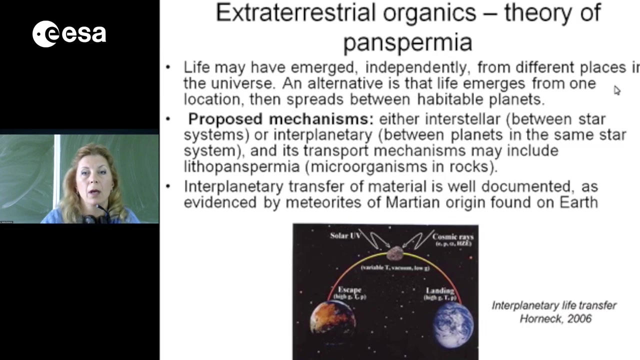 the surface or in underwater or wherever, or another way they could have arrived from outer space, which is an example of how it could have happened. And finally, we come to nucleic acids that currently are used as a carrier of genomic information. 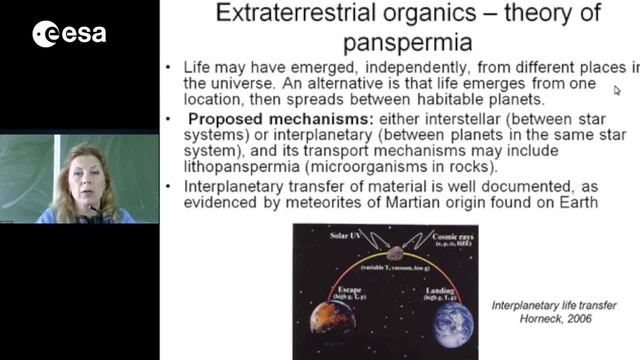 First of all, I would like to mention the theory of panspermia, which presumes that there are many different mechanisms for the transfer of material from one location to another, and that means that there are many different mechanisms for the transfer of material from. 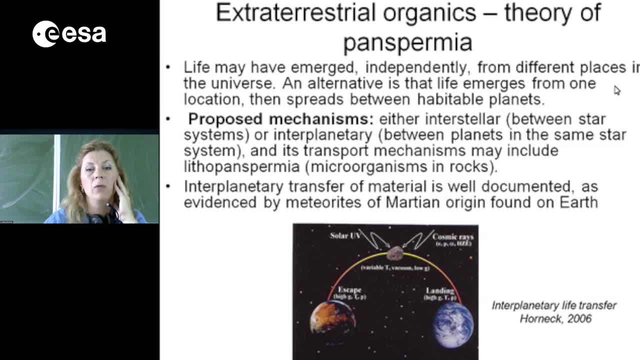 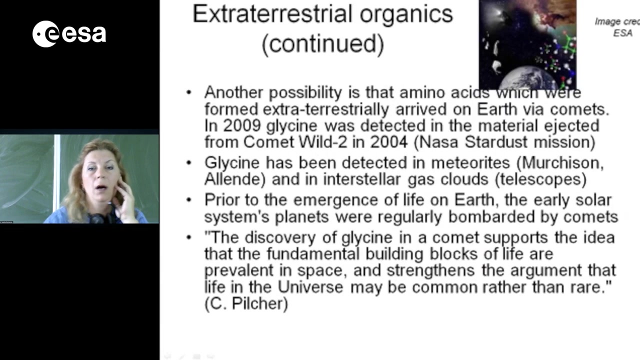 another place. For example, we have small carriers which travel in the solar system or in the outside universe And we have good proof that there is an exchange of material in the solar system and that is very important for the transfer of material from one 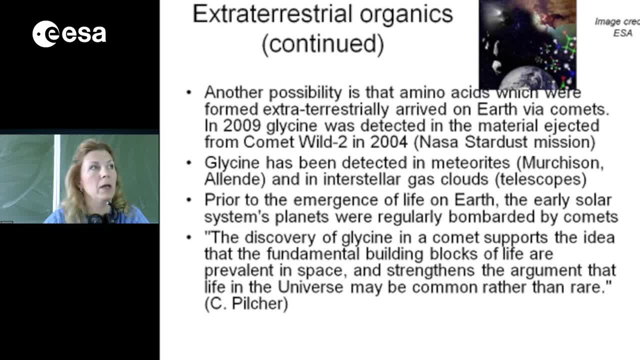 location to another. Another possibility is that organic matter could be transported by the solar system Also. glycine was detected in meteorites and in interstellar gas clouds. telescopic observations That means that organic material is quite common for the solar system at. 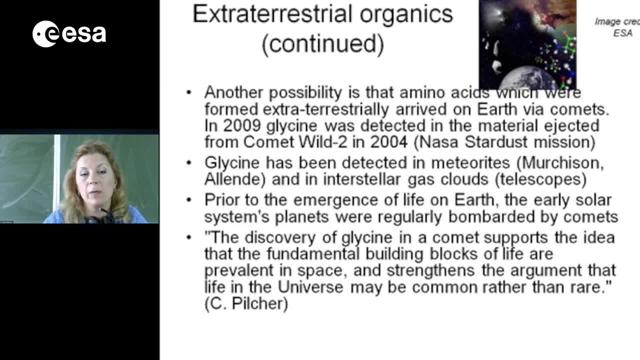 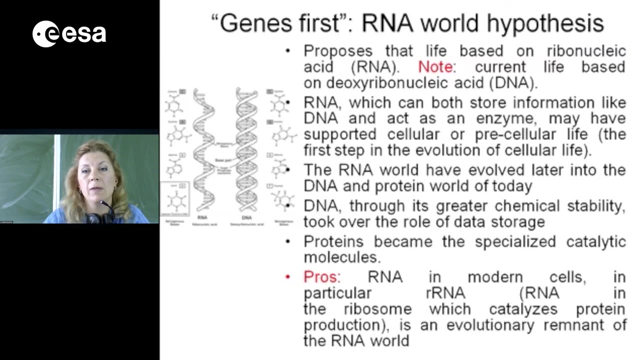 least in the solar system. This theory is quite plausible. Fundamental blocks of life are relevant in space and they could be carried by space carriers, Micrometeorites, which are falling in a big amount of the solar system, In the solar system. 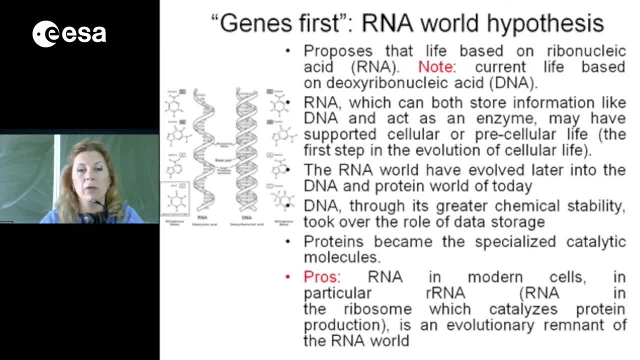 there are a number of molecules that can store information, like DNA, and act as an enzyme to perform self catalytic processes. In the world of today, And meanwhile in the time frame, DNA, which has better chemical stability, just overtook the role. 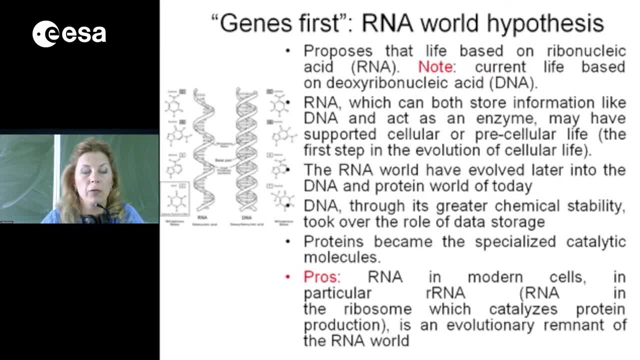 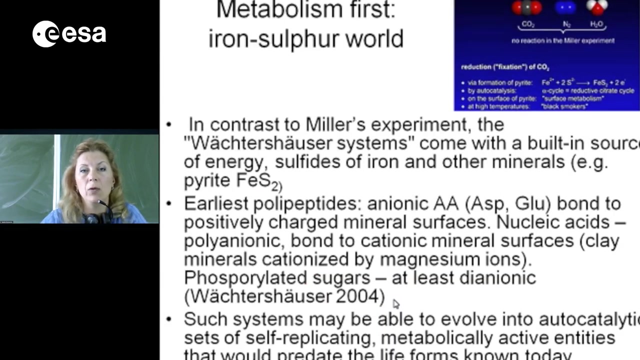 of data storage. One point that can prove the role of DNA in the world is that the DNA in the human cells are ribosome RNA. This is the RNA in ribosome which catalyzes protein production. So this is supposed to be an. 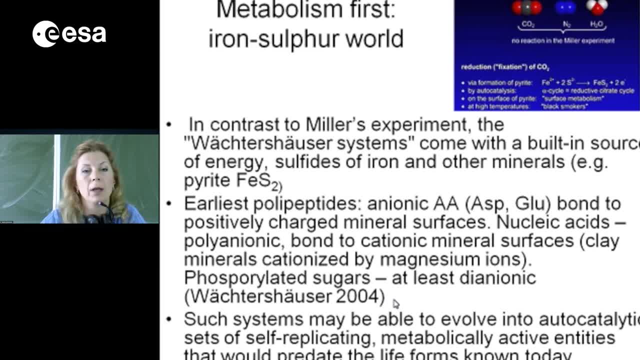 enzyme that is responsible for the production of new proteins. So it is an enzyme that is responsible for the production of new proteins And it is responsible for the production of new proteins, including pyrite, so derivatives of iris And those mineral surfaces. 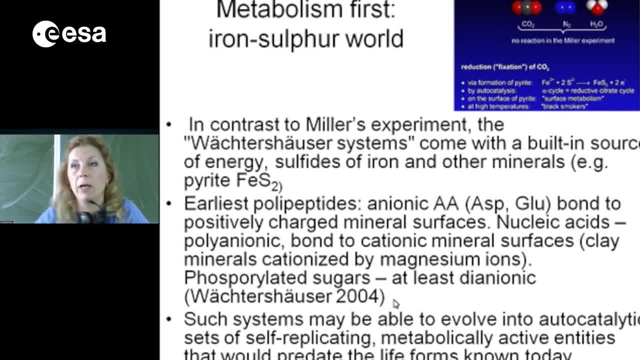 non-organic surfaces could be used as certain metrics for the formation of organic molecules, such as nucleic acids, that are used to keep the system together and serve both as catalysers and sources of energy. So if such system could be established, 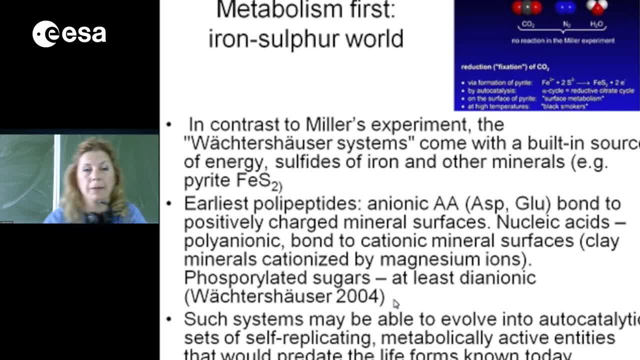 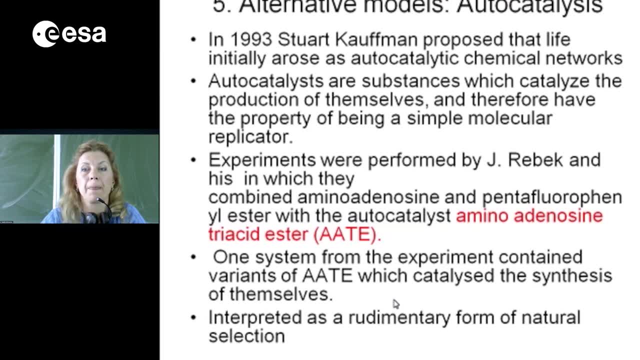 it was able to evolve later on with auto catalysis. So the idea is that life initially appeared as auto catalytic chemical networks, For example. auto catalysis are such substances that can produce themselves and can be a sort of chemical material. So if 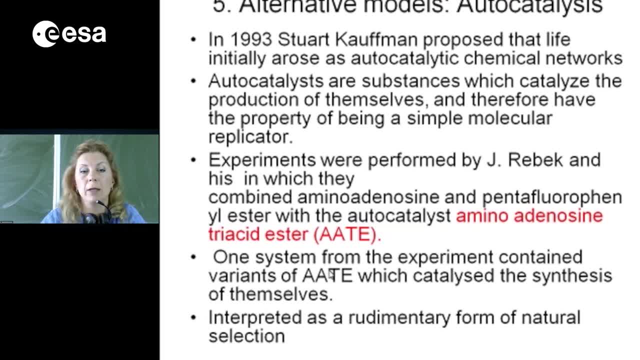 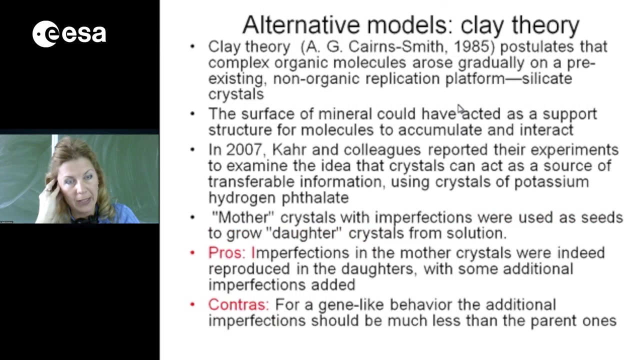 you look at this slide, you can see that there are a number of chemical structures in the system. So if such chemical structures existed during the early Earth, that means that they could take part in. they could evolve later on into chemical systems that we 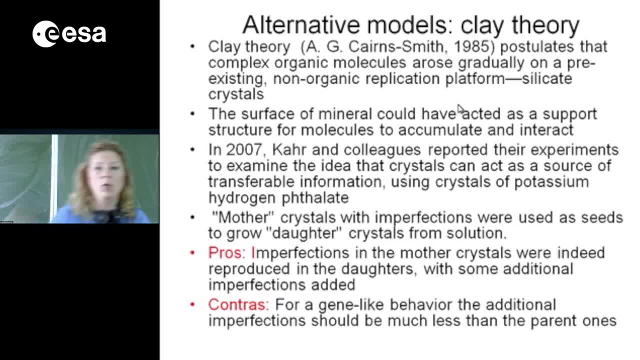 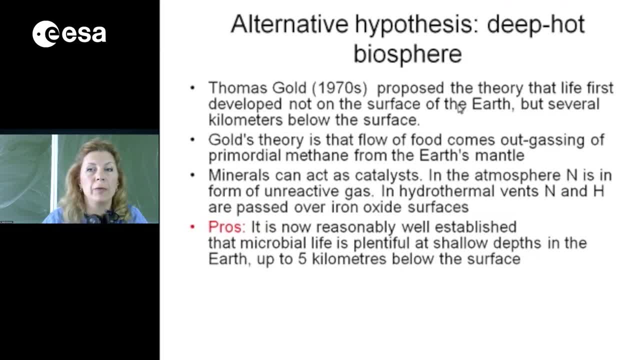 earth. if you take a look at the surface of the earth, you will see that the surface of the Earth is very like this place on the planet, Like the sun. So what we come to, the very catalyst, and there are a lot of organic material which is available on the. 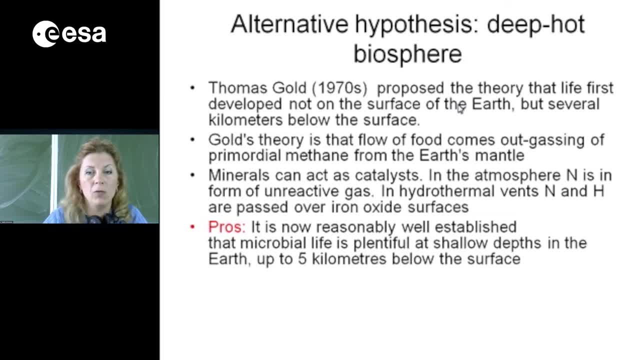 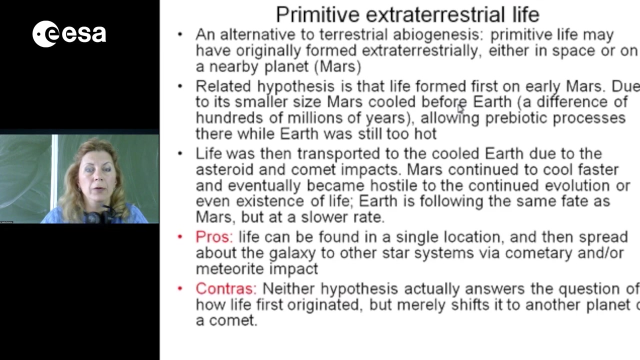 underwater level, so it can be used as a material for formation of complex molecules, and it is now well known that there is a big and big variety of microbial life under the water up to five kilometers below the surface of the ocean. so, if not to think how it appeared, we may think that there is an 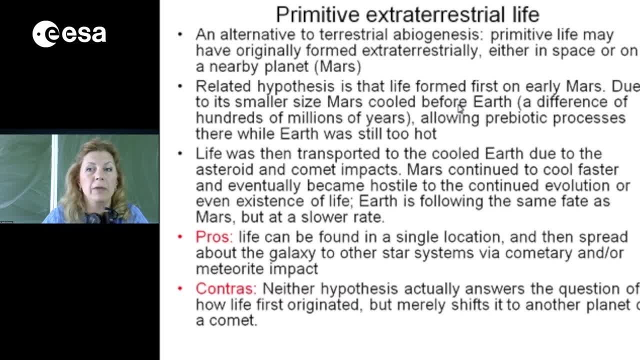 alternative to terrestrial abiogenesis. so primitive life may appear only extraterrestrially in space or on planets, and one of the hypotheses is that life formed first on early Mars and Mars cooled before Earth and the prebiotic processes could take place on Mars and at that. 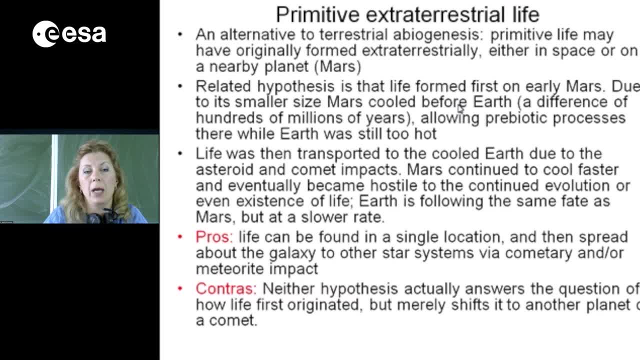 time our planet was still too hot, and then life was transported to the earth by comets and asteroids. so that means that life can be found in single location and then spread all around about the galaxy. but none of this has been discovered yet Actually actually answers the question of how life first originated. 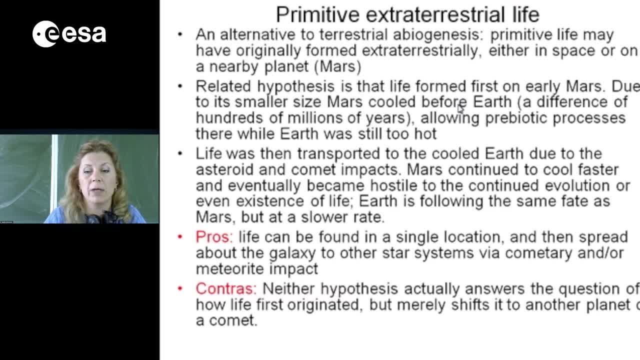 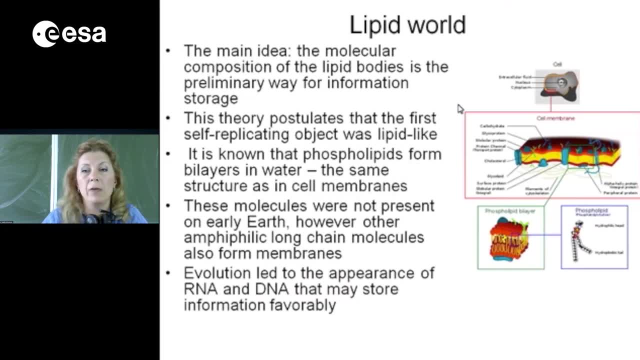 but sometimes it's just shifted from another location, from one to another location, planet or comet. Then I promised to say a couple words about lipid world, because lipids are important components of the cellular structure, so the idea that molecular composition of lipid bodies is also can serve as an information storage, and this theory postulates that. 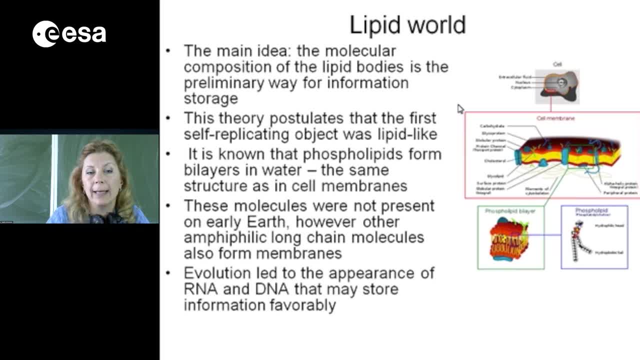 the first self replicating objects was lipid-like. It's very plausible because phospholipids form by layers in water very easy and it has the same structure as cell membranes. we should mind that these molecules were not present on early Earth, but there were other very long chain molecules and they had collided reaction to the germ's being formed on the earth. 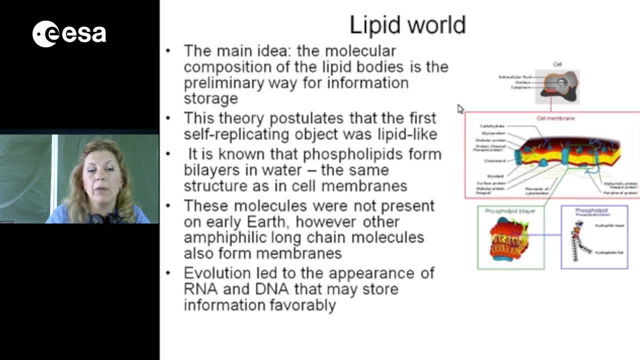 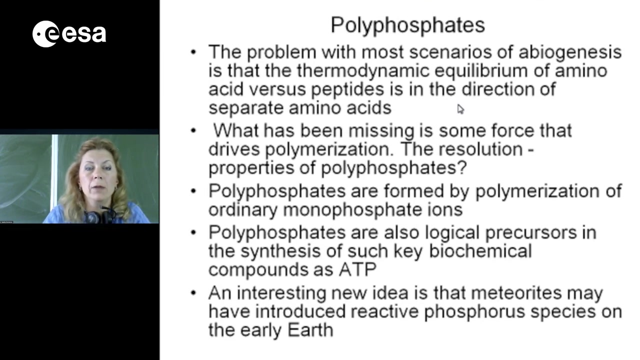 amphiphilic who could, who were able to form membranes, as nowadays we know that evolution led to the appearance of DNA and RNA that can store information much better than any lipid. but when RNA and DNA is not available, this function may be attributed to lipids. so all of us fade the problem of the most scenarios. 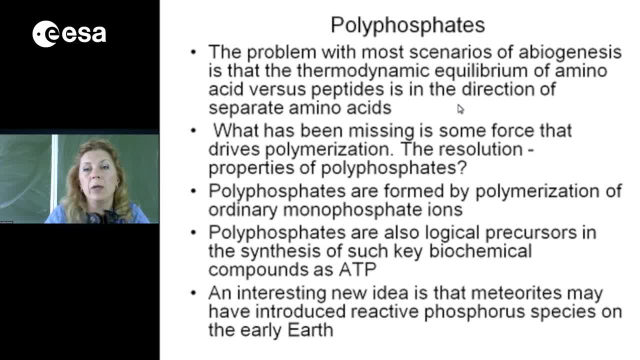 is that we have thermodynamic equilibrium and the the. this equilibrium favors the separation of amino acids, not the formation of long molecules. some, there should be some force. force that could drive the polymerization to help shape up long molecule could be the resolution or in properties of. 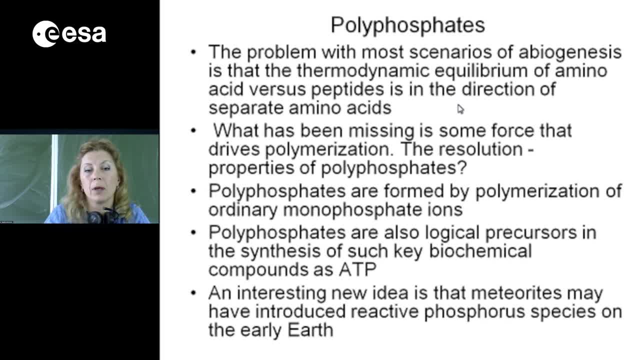 polyphosphates. polyphosphates are formed by polymerization and also they can be precursors in the synthesis of such key biochemical compounds as ATP, adenosine 3-phosphate. so it's included and it's used as an energy storage. so if 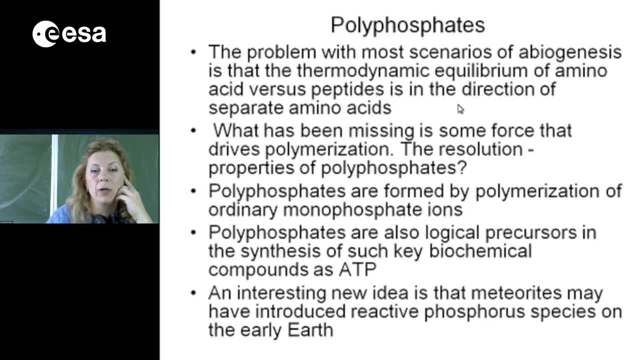 you if to use the chemical energy stored in polyphosphate. maybe this is the case, but if you want to use the chemical energy stored in polyphosphate, maybe this can help to move the equilibrium to the side of formation: long chain, long polyphosphates. 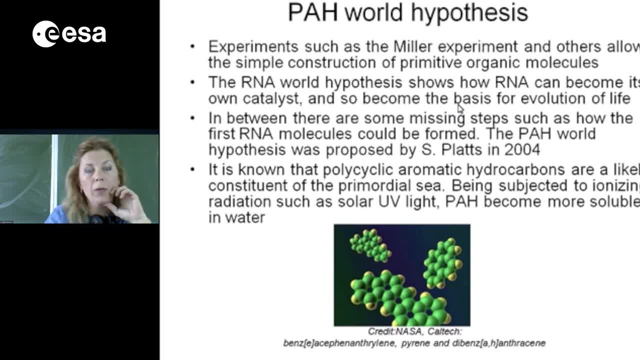 then they were also certain ideas and hypothesis that include included: polycyclic aromatic hydrocarbons, which are quite interesting substances, helping obtain certain properties, certain qualities. polycyclic aromatic hydrocarbons, which are quite interesting substances, helping obtain certain properties, certain qualities. There are some missing steps that are not included in RNA theory, which are considered. 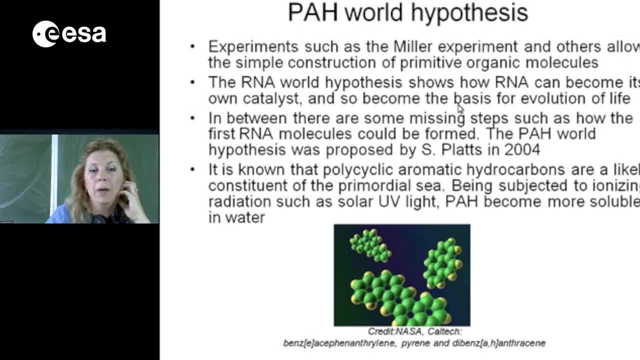 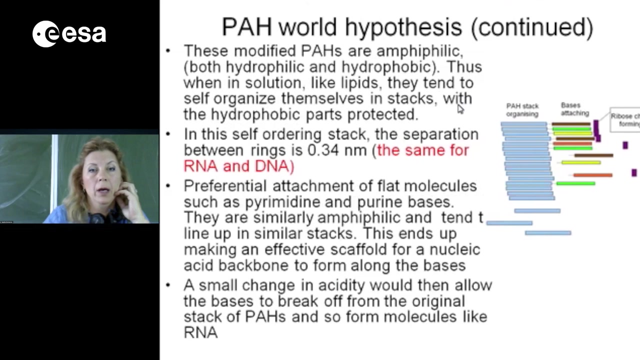 in the theory of PAH, They are likely the constituents of the primordial C. They were present at the primordial C. And these substances, these molecules, if they were treated by ionizing radiation, for example UV light, they can become more soluble in water. 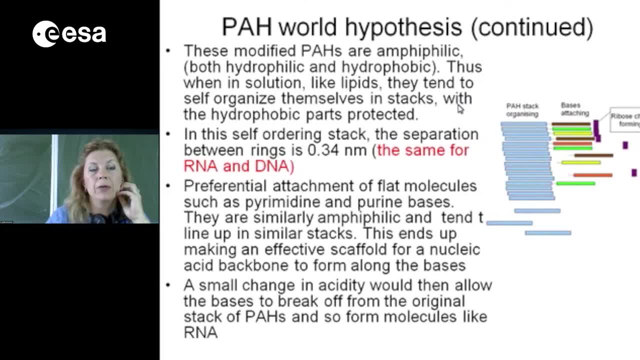 Being modified. they form like lipids, They self-organize in stacks And what is notable? that the separation between the strings, the distance between the stacks, is the same as in DNA, The distance between bases in DNA and RNA. So if we have in the same solution molecules of pyrimidine and purine, for example, they 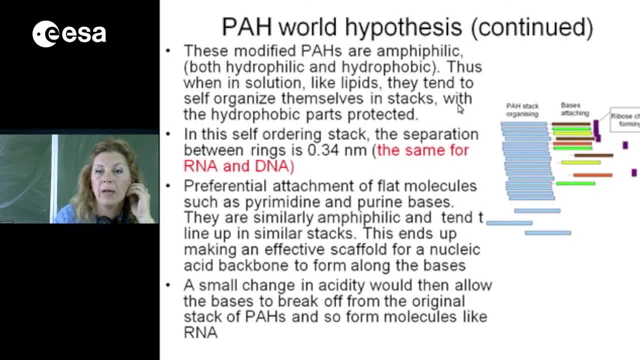 can connect with this PAH stack organizing and then the ribose chain can be formed. additionally, Having this structure, we need just to dissolve it. So small change in acidity it can let the bases to break off from the original stack and to form molecules like RNA. so this is quite nice explanation of how. 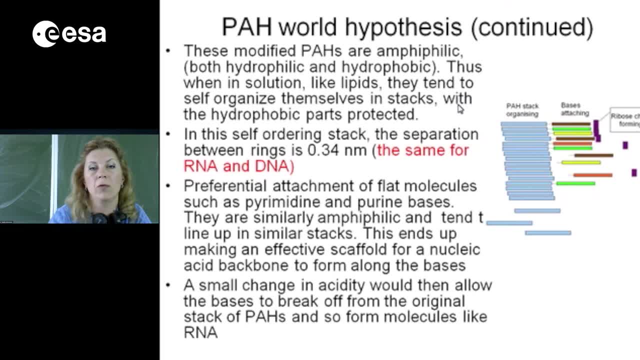 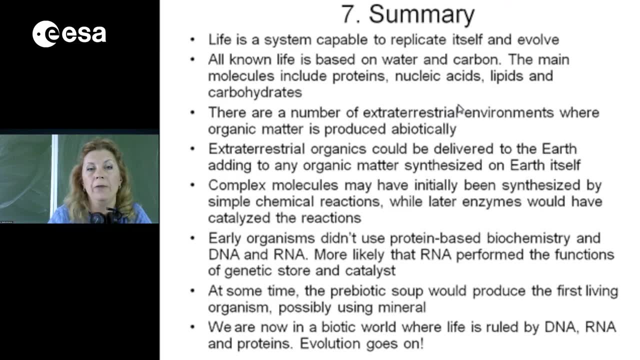 structurally RNA molecule could be formed. so let me give you a brief summary of what I try to tell you. first of all, life is a system capable of replicate and evolve. we told it from the very beginning. we know that all known life in present is based on water and carbon. main molecules include proteins. 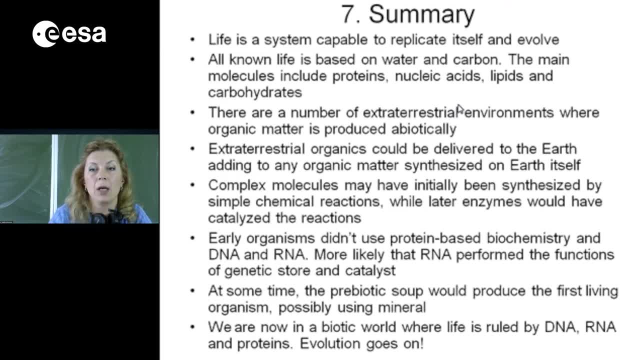 nucleic acids, lipids and carbohydrates. we should consider a number of extraterrestrial environment, environment where organic matter is produced, and if it is produced externally, then it should be somehow delivered to the earth or to any other place. in general, in general, every theory presumes. 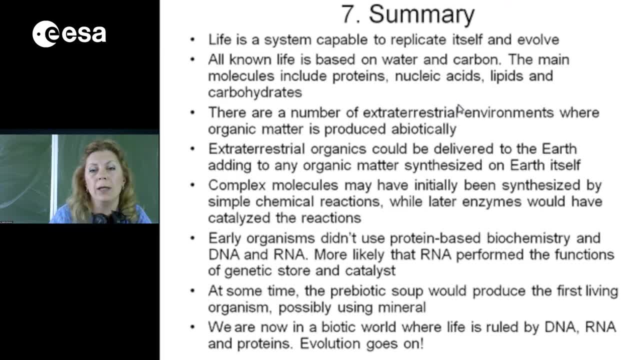 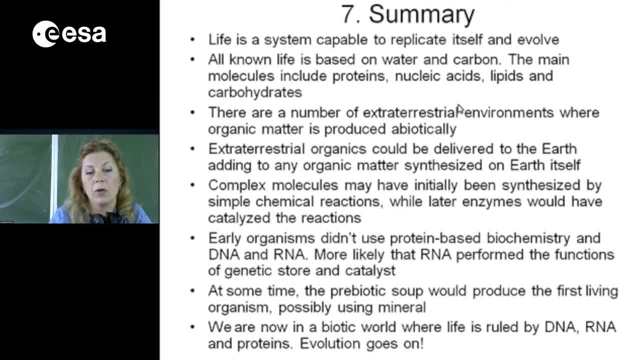 happens, the prebiotic soup, which is the liquid environment, uh would-produce the first living organisms. possibly you using magical matrices as it was shown in them, theory's including organic and non-organic materials, and right now we are innotic. world and life is ruled by DNA, RNA and protein. 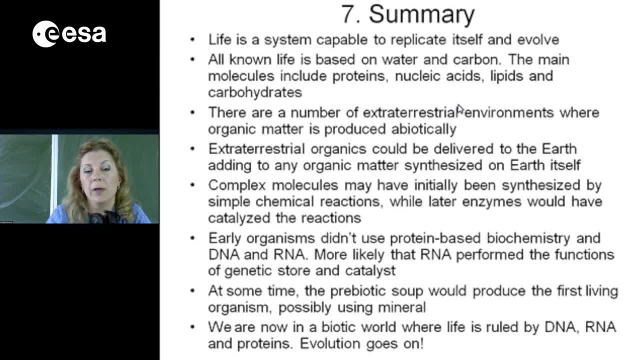 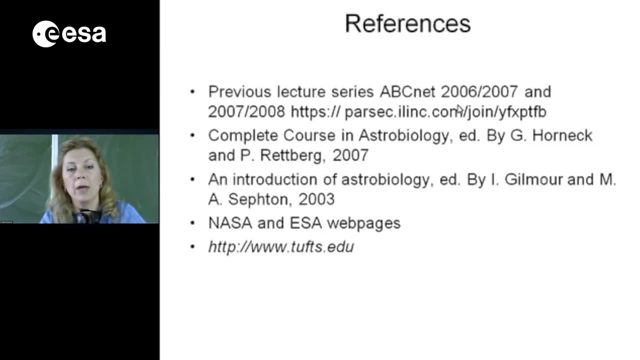 but that doesn't mean that everything stopped. evolution goes on. so we have evolution of human mind and this is another step. okay, so here are the references. I'm sorry, I think that some of these pages were removed, but still. we have the books of complete course on astrobiology and introduction of 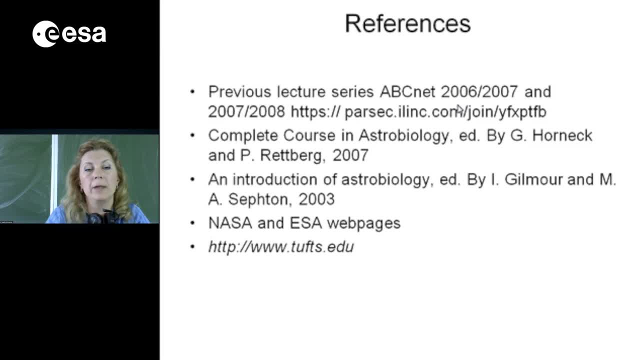 astrobiology. if you surf the web, you will find a number of materials related to this idea, to this topic, and mostly the NASA and ESA web pages. they have separate- I left- I'm wrong- out of words. okay, you just see there is a lot of information given there on all the subjects that I mentioned. 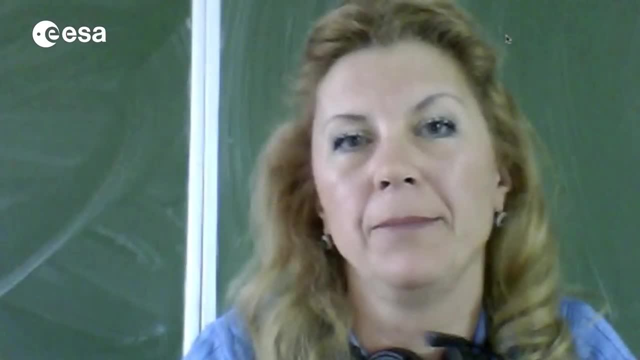 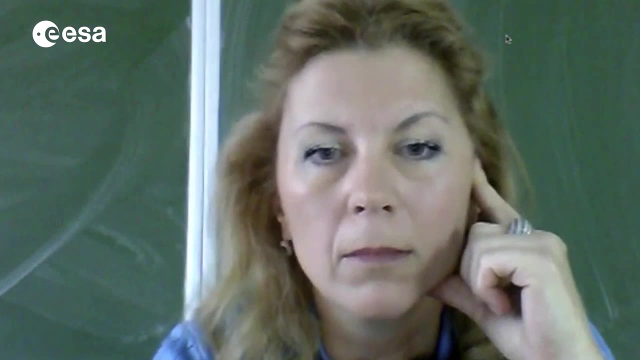 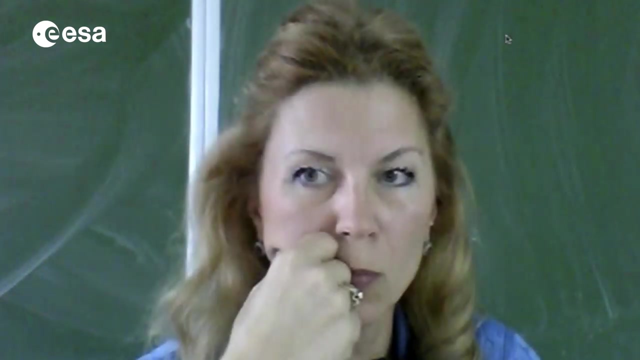 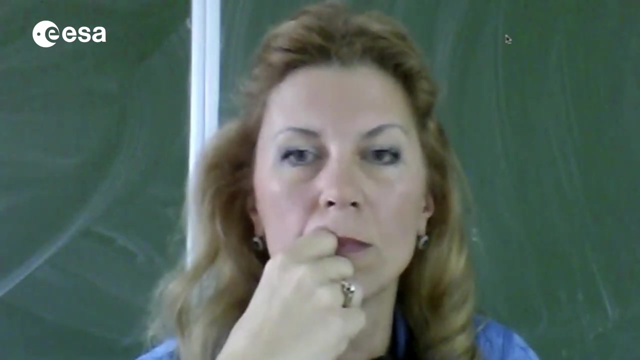 thank you. thank you for your attention for Alessandra. Alessandra from the University of Napoli. I see that you're back, is there? are there any questions? just just a second, because of the city. ah, he would like to know a bit more on the air. and a hypothesis: 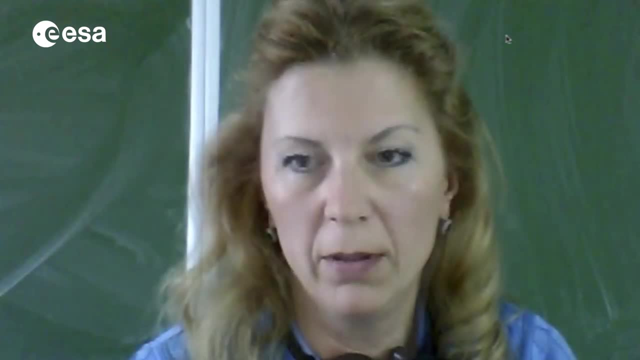 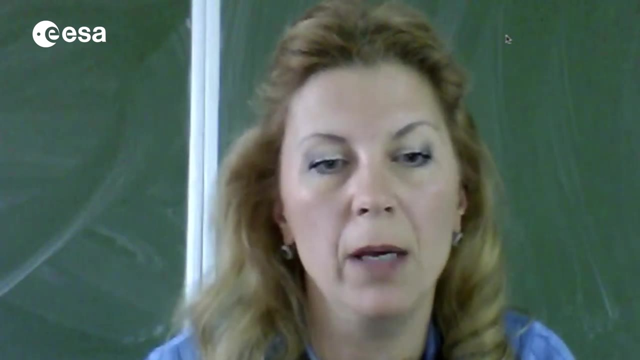 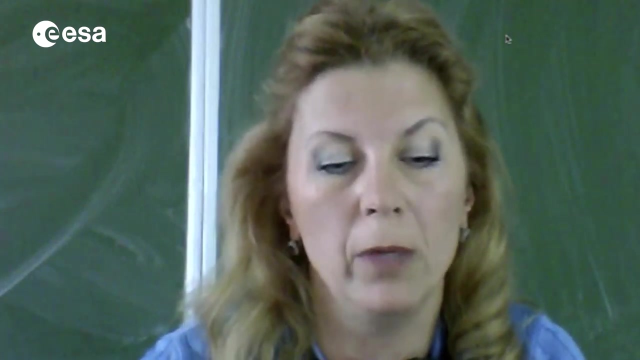 airing a word hypothesis, yes, okay, so I mean, RNA world is such a great area, it's a big question with a lot of details. that I'm. I think I'm just unable to cover the subject within frames of our lecture and also in one question, but I 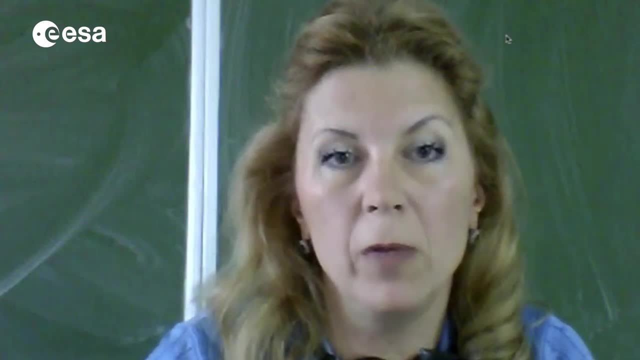 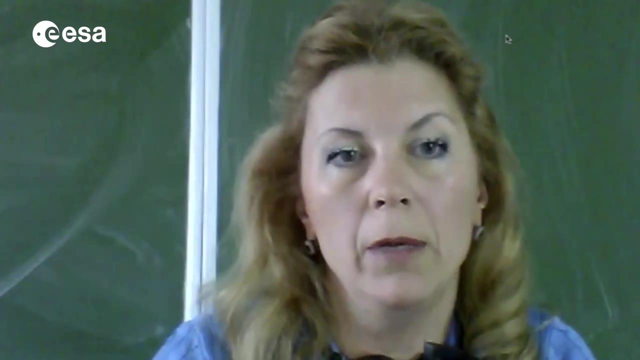 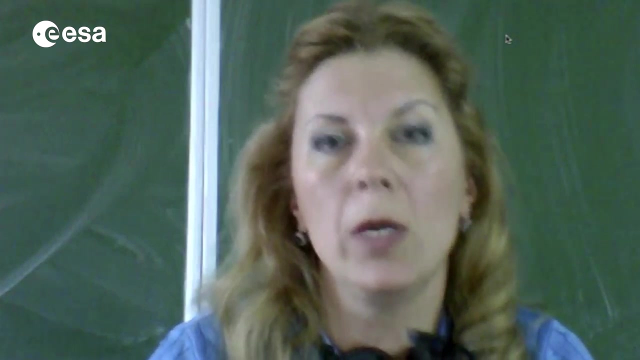 would say that currently it's one of the most popular and popular topics in the important theory, which is well-proved, and there is a lot of information, a certain type of experiments carried on. so I think that if there are certain details that I interested, that you are interested in, you may easily find it in. 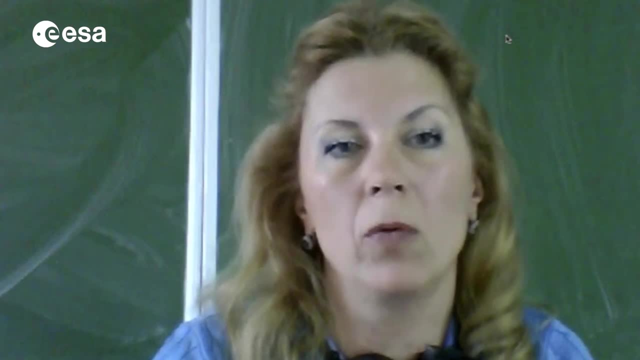 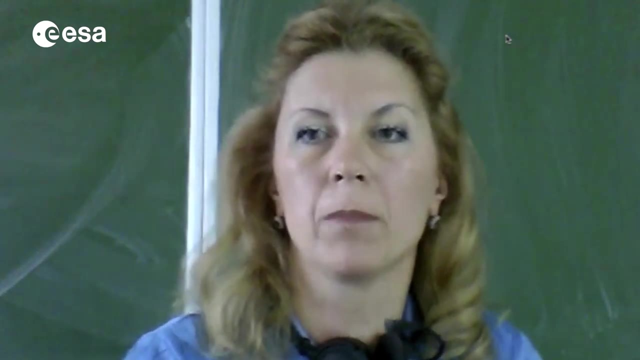 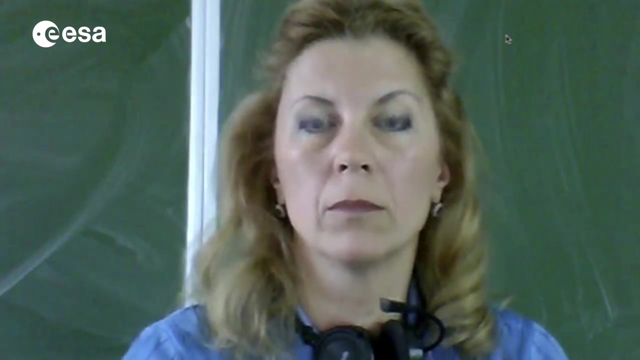 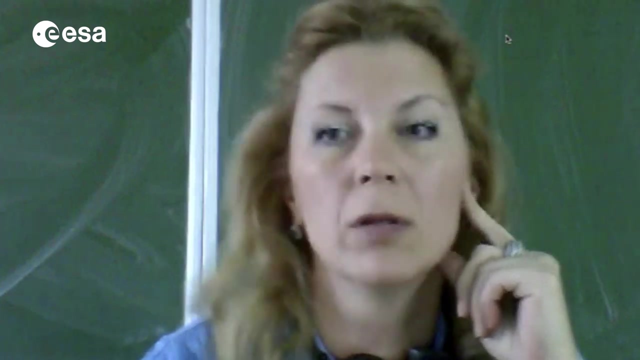 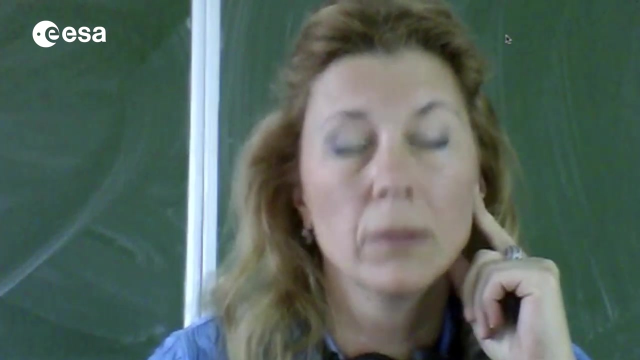 the internet, or in their libraries or everywhere. so this theory is quite known. that that's my message. okay, I will pass now to University of Turku. are there any questions from from there? hello, can you hear us? okay, okay, okay, one question, Natalia. thank you for introducing this very complex and complicated issue. I 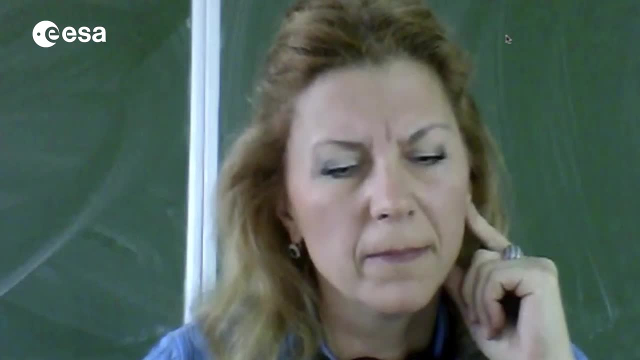 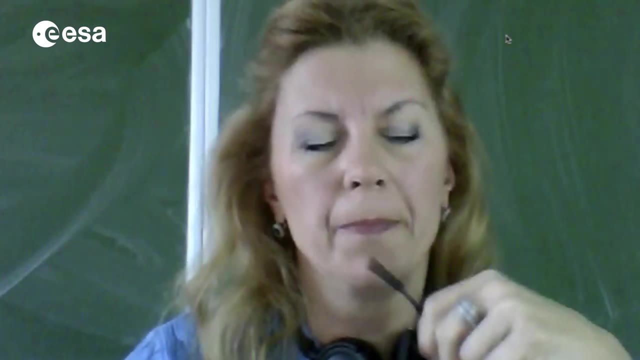 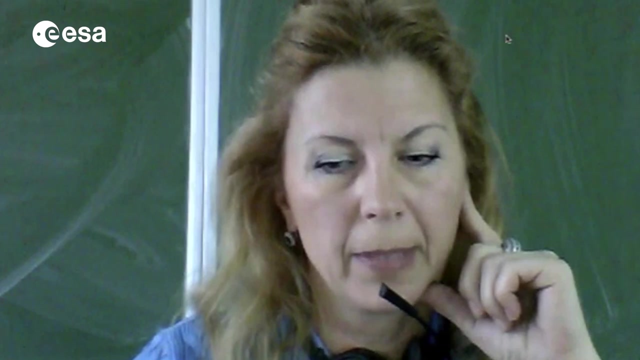 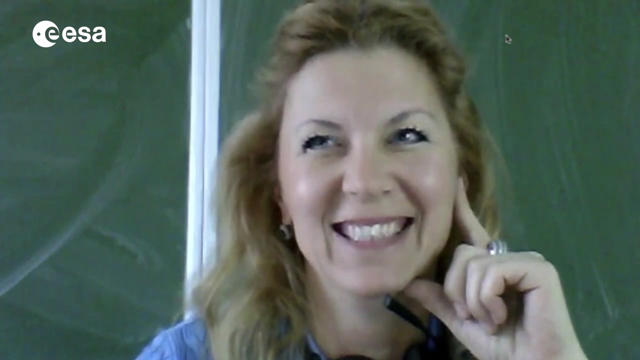 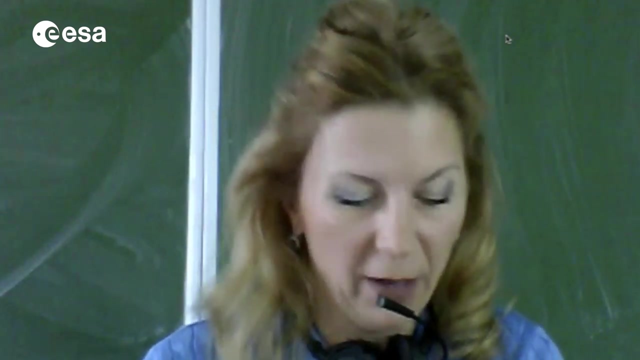 would like to ask of: can you give some kind of a overall sequence of events that has taken place in the transition from the prebiotic chemistry to the first real living organism? so what kind of things have to happen or what kind of process? so, Kirsti, which which is 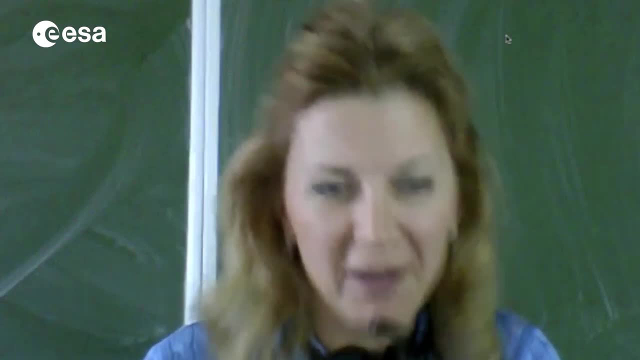 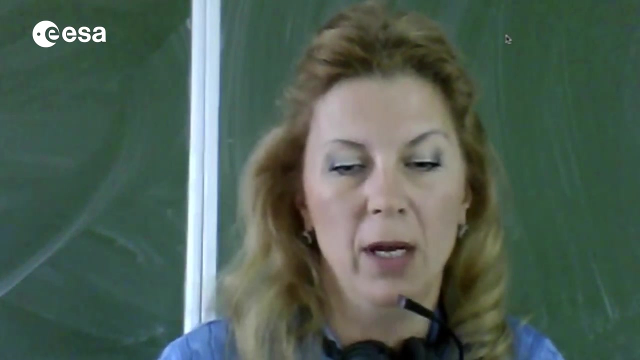 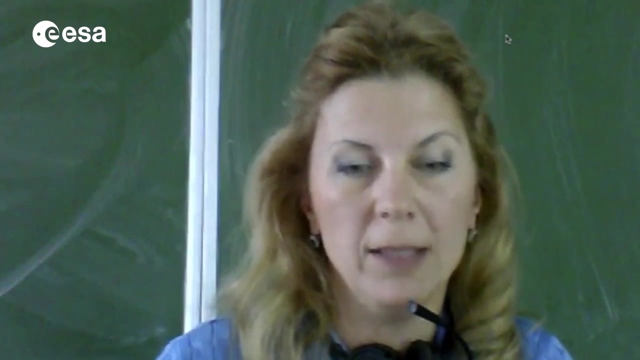 quite clever, I would say, and with a different knowledge in all kind of areas. she definitely knows that this question is a weak point of the whole evolution theory, of the whole evolution process. so it's right. now it's more or less understandable how basic molecules proceeded to to. 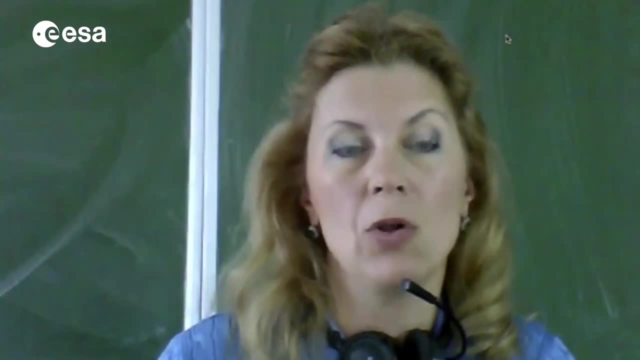 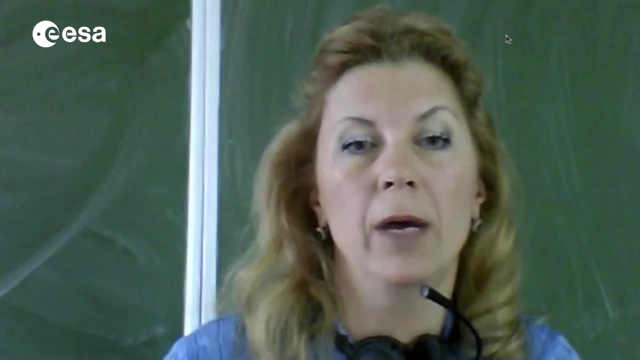 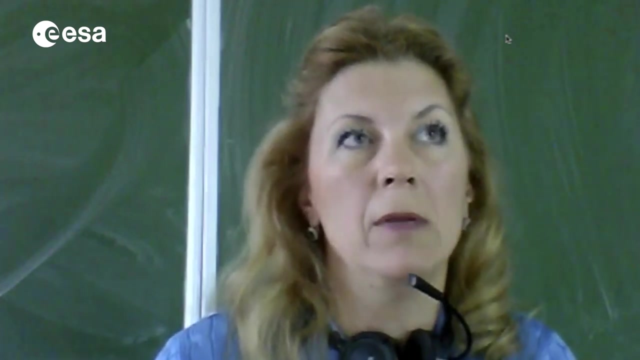 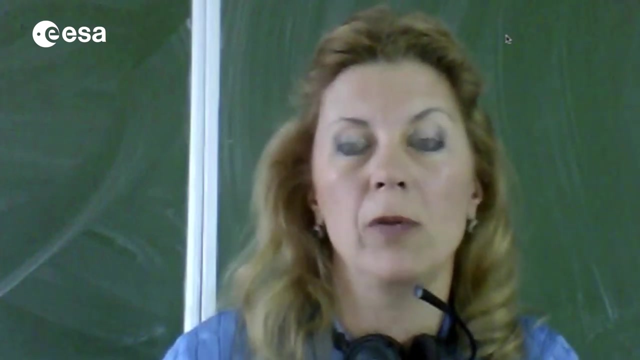 more complex molecules. but we should, um, we should presume that no one so far was able to construct, uh, first living cells. so there is a gap, theoretical and experimental, in this evolution scale, in between complex molecules evolving, reproducing, making everything, but still they were not, we were not able, i mean the whole, the whole mankind was not able to construct first. 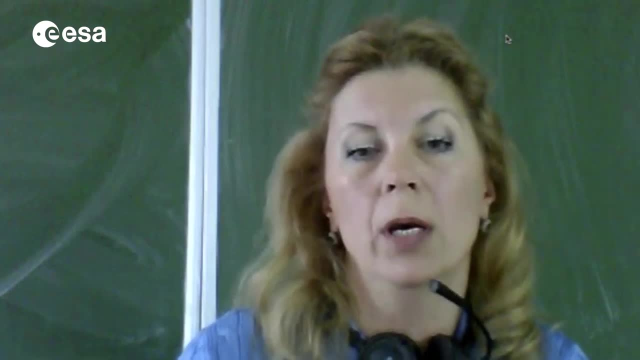 living cell functioning in vitro and there are certain questions of how, how it, what happened before it appeared? so it could not appear spontaneously. there were certain processes that led to it, but so far it's not, it's not yet clear. okay, i i have one question, one comment. 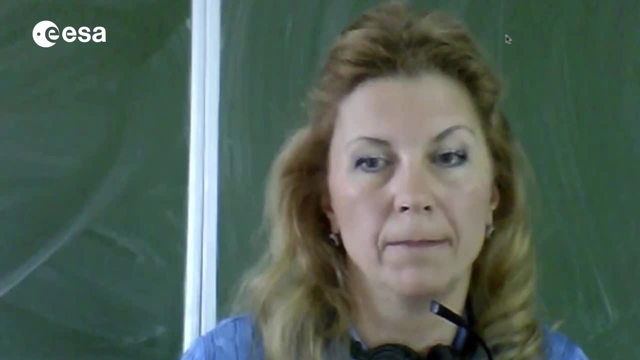 uh, first of all, the sun about four billion years ago was fainter than now. it's believed to have been about 30 percent, and if you consider the distance to mars, it's about twice the distance than what earth is from the sun. this means that that mars received only an energy amount which is 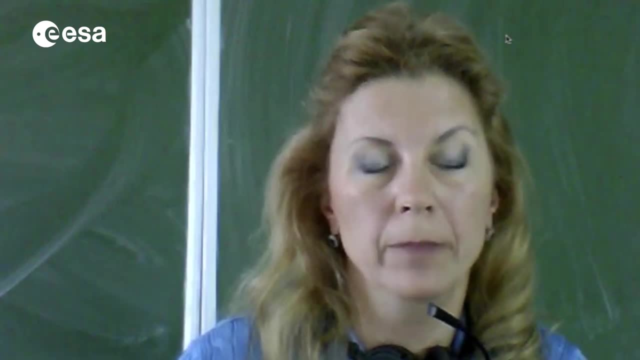 15 percent of the present value. if you turn this into numbers and calculate the temperature of the mars, you get something like 150 kelvins. this means that in order for life to emerge and to water stay in liquid form, you would have to have a greenhouse. 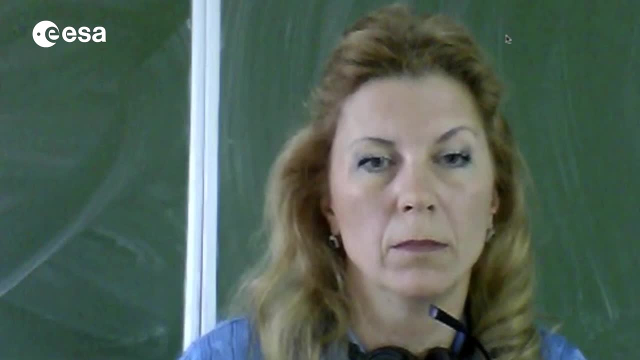 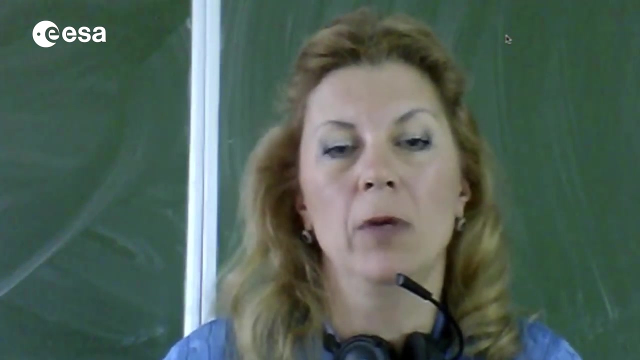 effect, which is about 100 degrees. so that's that's quite a lot. yeah, do you have any ideas how we could have a 100 degree greenhouse effect? it's three times more than what we have on the earth right now. so you mean that on mars there were not enough energy in general at that time to start chemical. 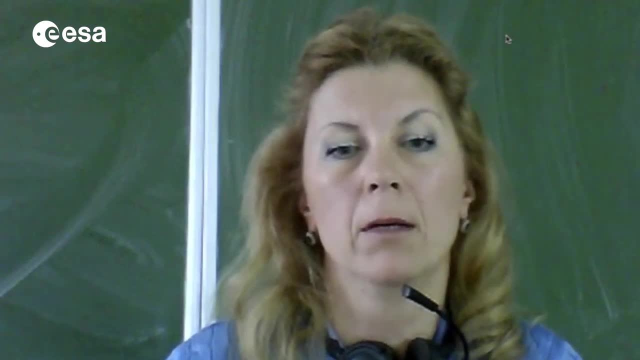 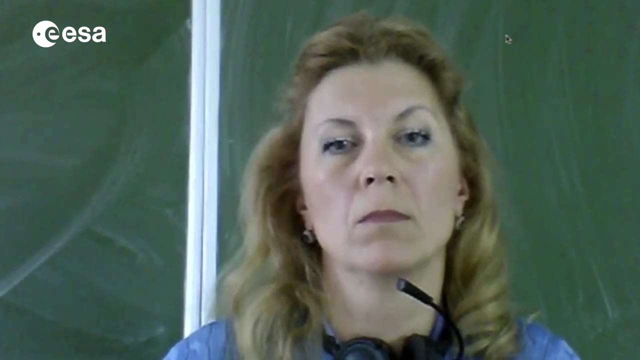 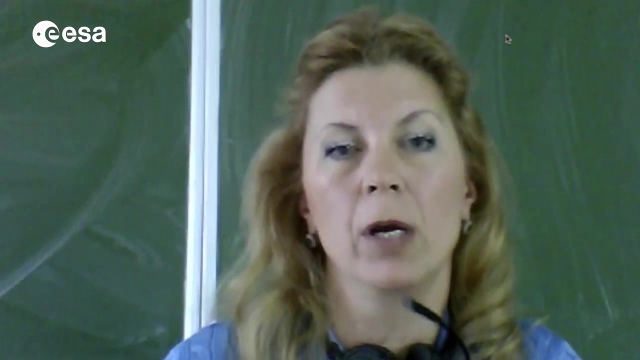 processes. uh, there could have been enough of energy, but you need a huge greenhouse effect to warm the surface so that water stays liquid there. okay, so there were not enough um prerequisites, basic conditions for uh life to start on mars. that that's, that's what? yeah, that's. 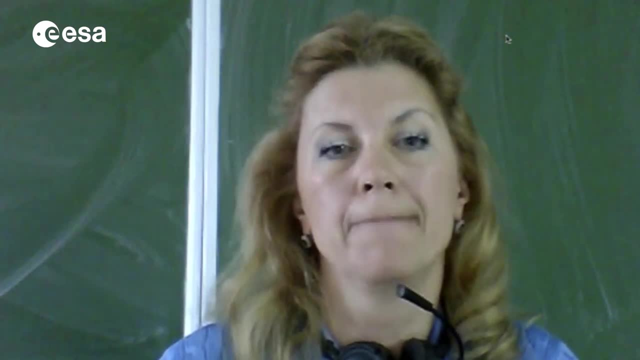 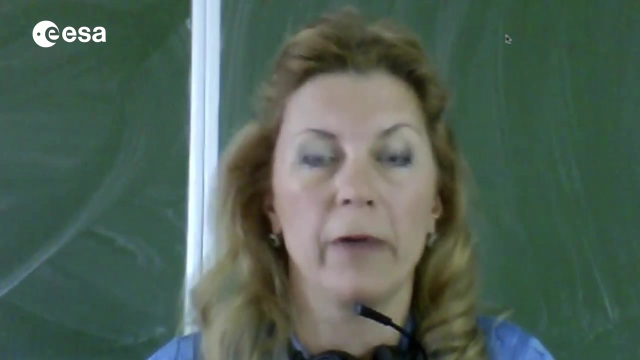 one thing that we we have to consider seriously: how to get it. well, uh, maybe in early days the situation was different and mars was warmer than the earth, or could be that some other situation on the primitive mars was different from, was more favorable, i would say, and in general more favorable, and also, to my mind, the martian atmosphere. 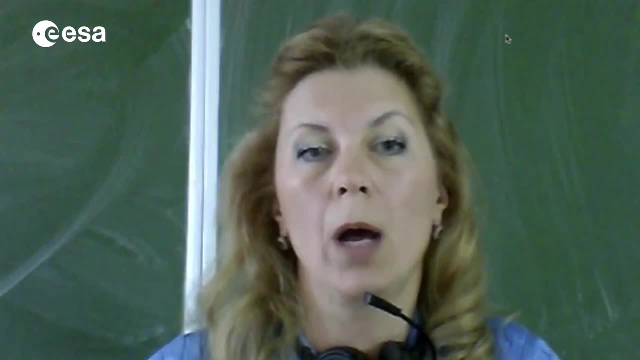 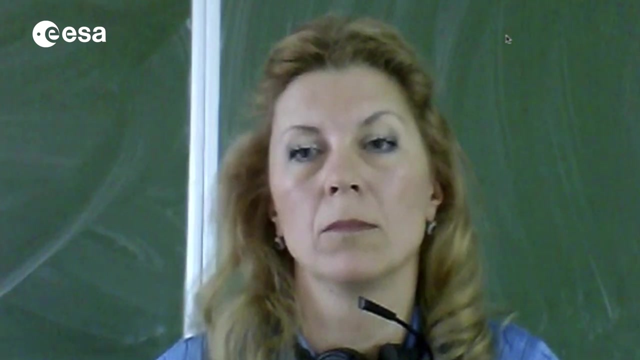 was much weaker than terrestrial, so i would say that external energy was able to penetrate to the surface better than uh on earth, so that could provide an extra energy for chemical processes to start. okay then, then i i have a short comment about about uh panspermia. as you mentioned, panspermia is 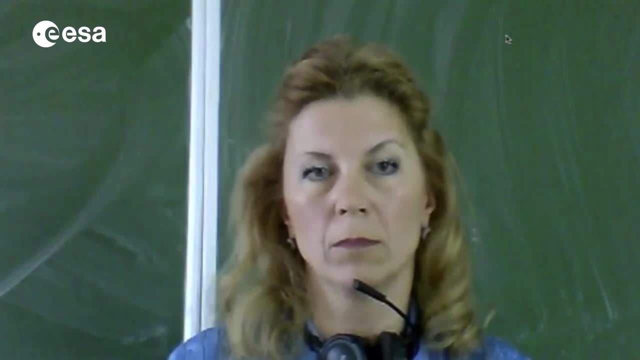 very different, but there is a lot of Tabitha, or, as you said, a way of describing it. so you mentioned solar systems. uh, and, and the way of describing something like that is actually that the problem with the solar system is that it's difficult to separate them and make a binary system. 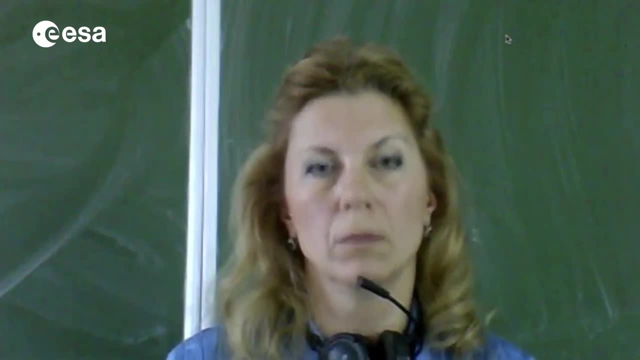 between between planets within our solar system, using asteroids, but not not comets, because comets are too fluffy. uh, and in. Okay, that's all from Turku, Thank you, Thank you, Harry. Okay, thank you, Harry, for those questions. Do we have any questions from the University of Szczecin in Poland? 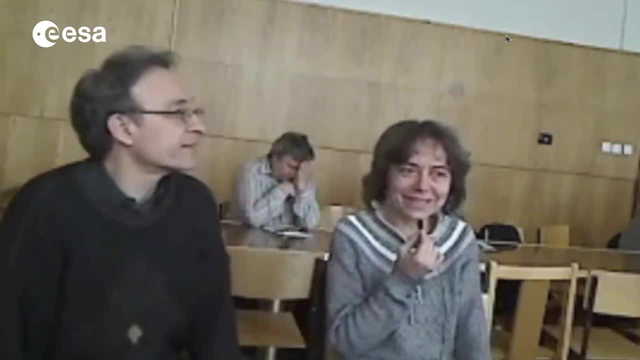 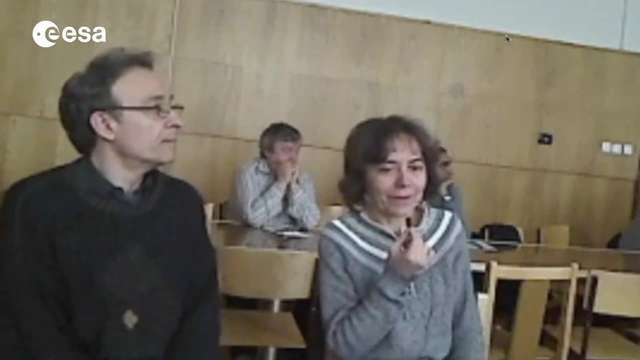 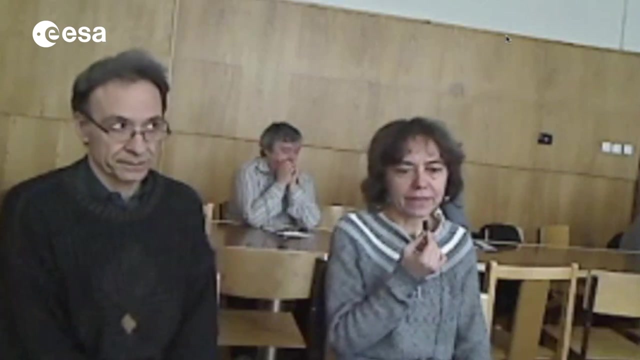 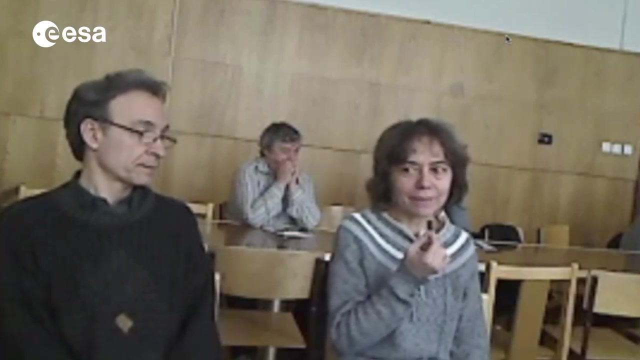 Thank you. Thanks for very interesting talks and I'm curious about the scenario for origin of life, I mean in the context of the energy which is used by the primitive organism at the very beginning. I mean it could happen, as you, Natalia, very nicely described. 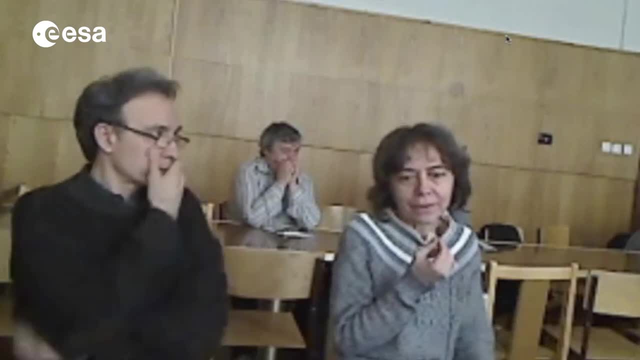 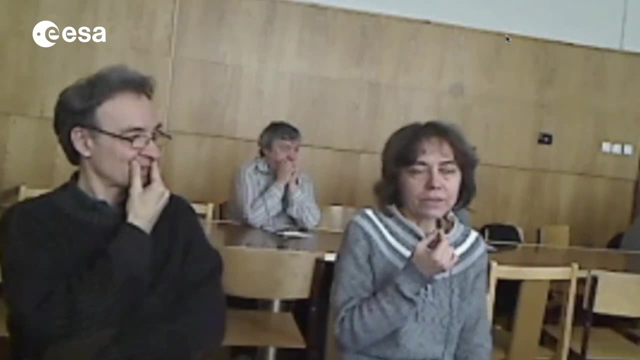 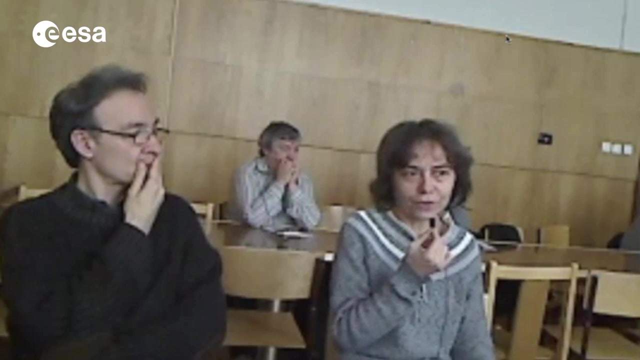 It could happen. I mean deep in the water, in ocean. It could happen also on the surface. So what is your feeling? I mean, which place is more important, Which place is more suitable for origin of life? I mean, if it's that, I mean the. 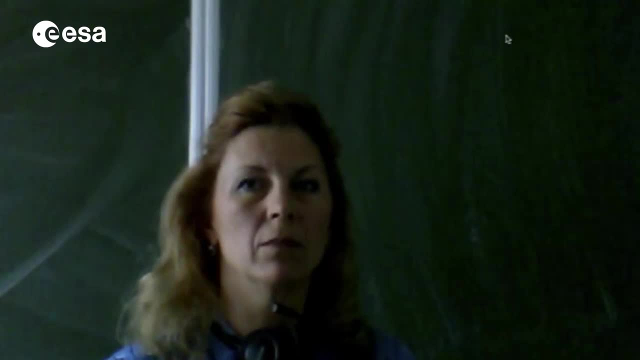 organism which are using chemical energy got some more preferences, or those who could already make use of the sunlight. So can you comment on that? I have a strong feeling that to make life appear in the natural environment is very important. I mean it's very important.